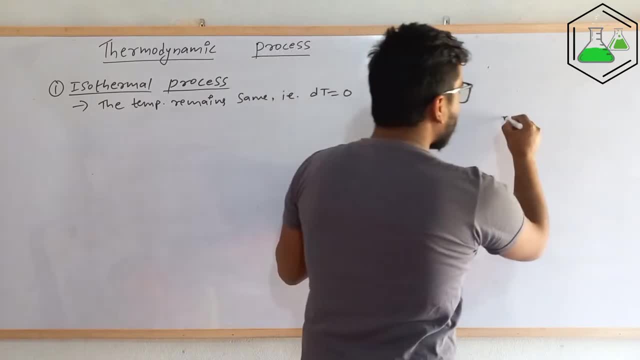 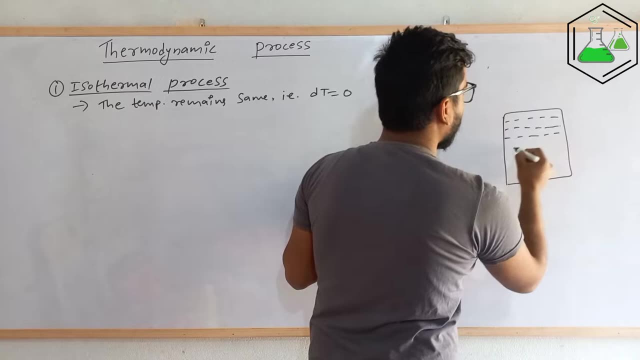 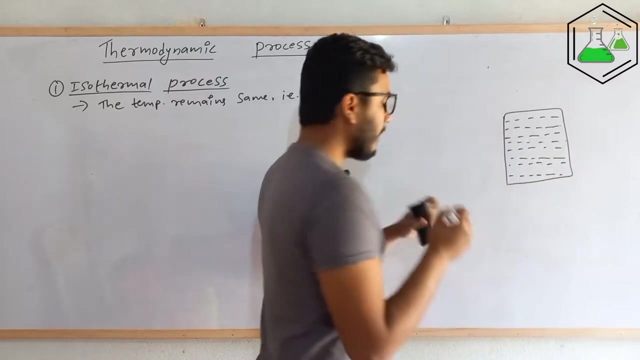 process happens in thermostat. okay, let us consider there is a thermostat in which the substance is put. this is the system, okay, okay, okay, see, I have told you the temperature should not change, but to maintain the temperature, there might be exchange of heat energy between the system and the 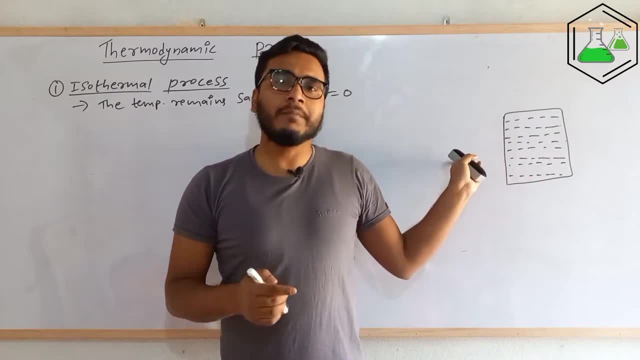 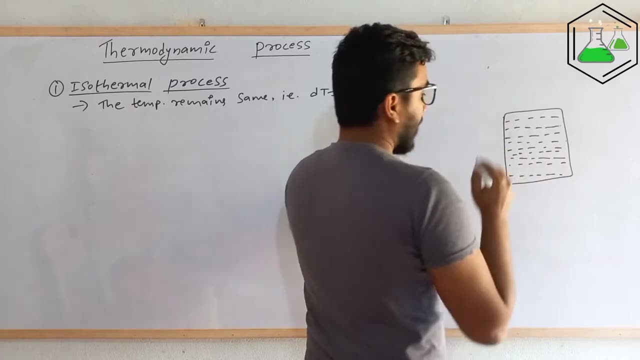 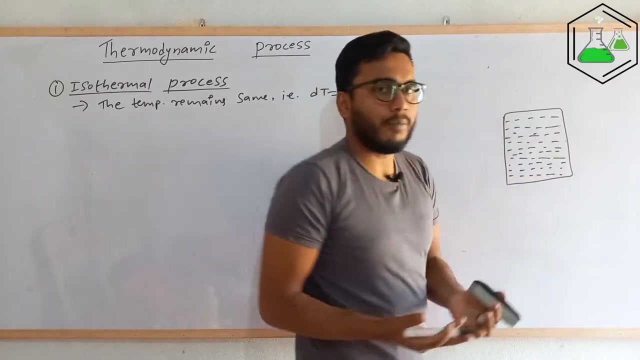 surrounding. okay, if you don't pay about system and surrounding, then please check the link in the description below. I have put the video over there. now, here the reaction is happening and suppose this is the exothermic reaction. then what happens? exothermic reaction means heat energy will produce in the reaction itself and 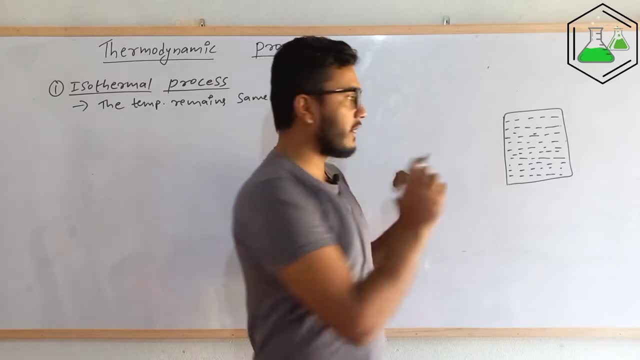 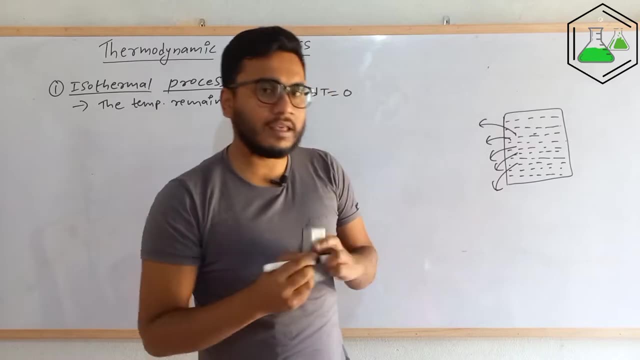 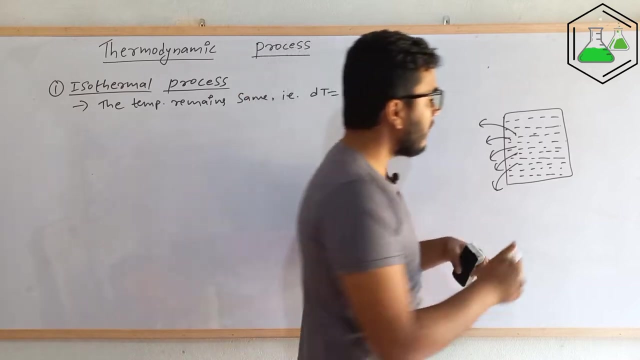 the temperature should increase. but to keep the temperature constant, the heat energy is absorbed by the surrounding. okay, the heat energy is absorbed by the surrounding to keep the temperature constant. in the another case, let us consider the reaction happening inside. the system is endothermic, now it 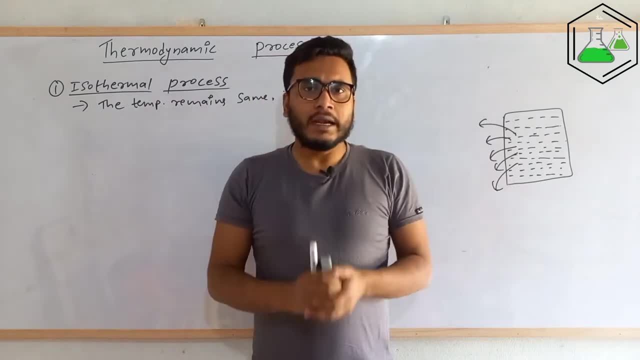 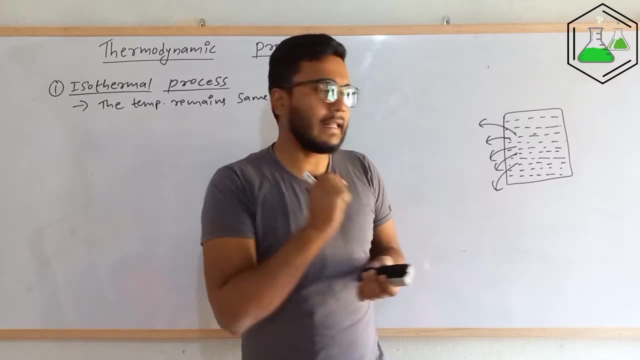 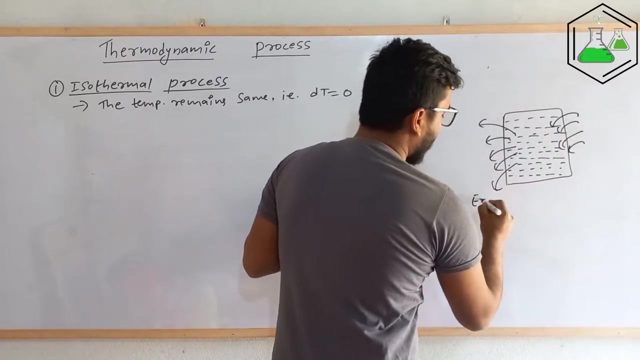 endothermic means obviously the temperature will decrease. now, in order to balance the temperature, it needs heat energy, and that heat energy is supplied by. yes, you are correct that heat energy is supplied by the surrounding. it is supplied by the surrounding. this is for exothermic, exothermic reaction and this. 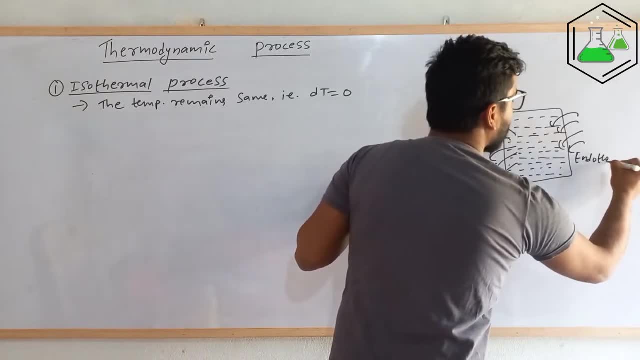 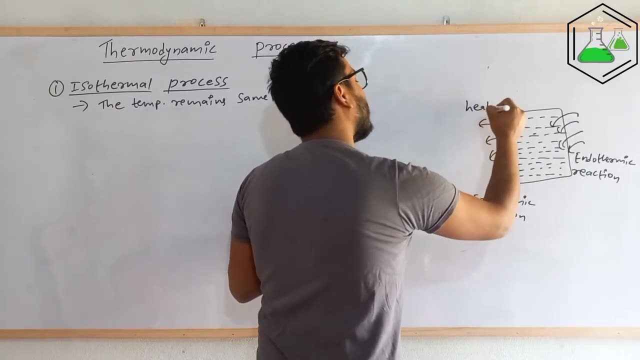 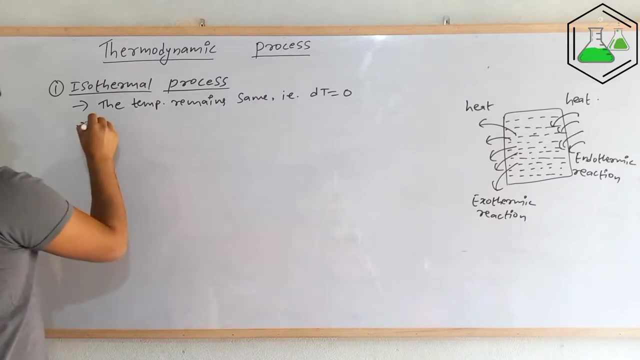 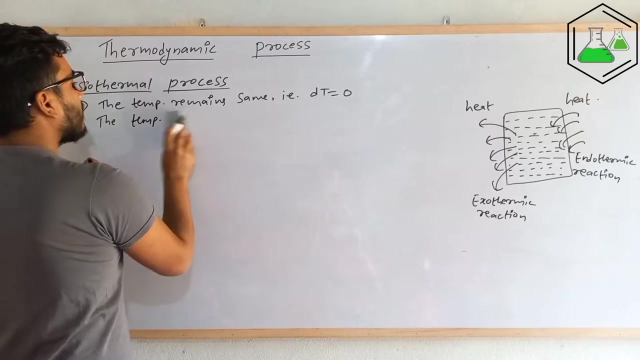 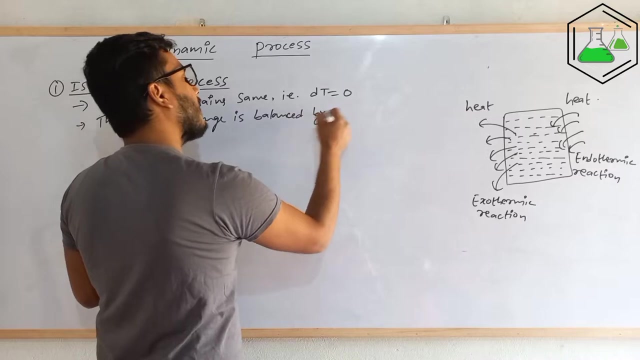 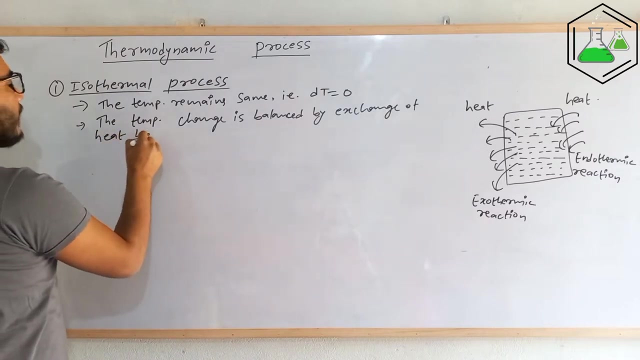 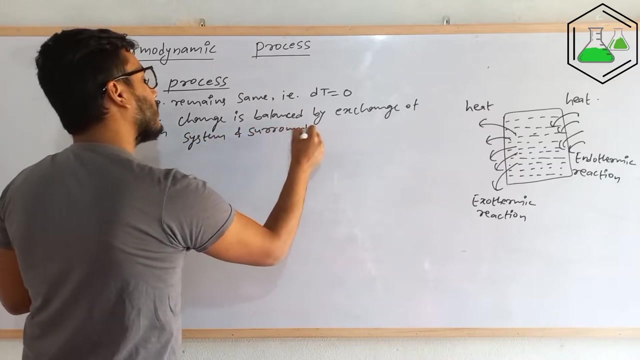 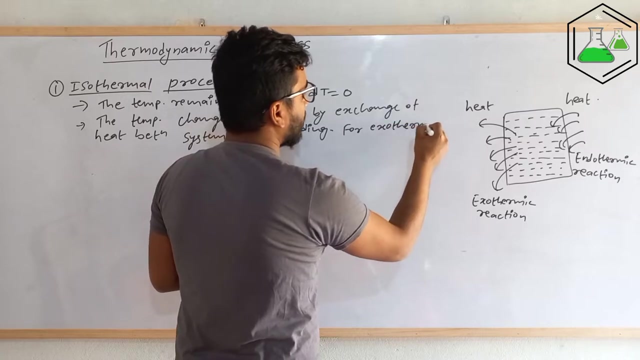 is for endothermic reaction. endothermic reaction, this is heat energy going out, this is heat energy coming in. okay, so let me write that over here. temperature, the temperature, the temperature change is balanced. balanced by exchange exchange of heat between between system and surrounding system and surrounding for exothermal, for exothermal process. 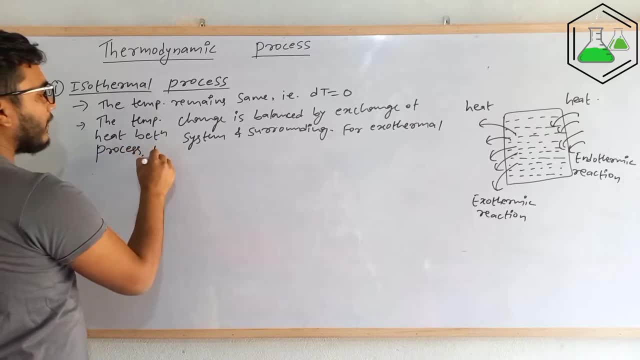 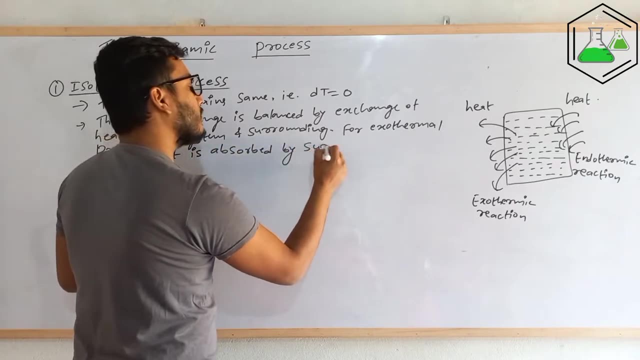 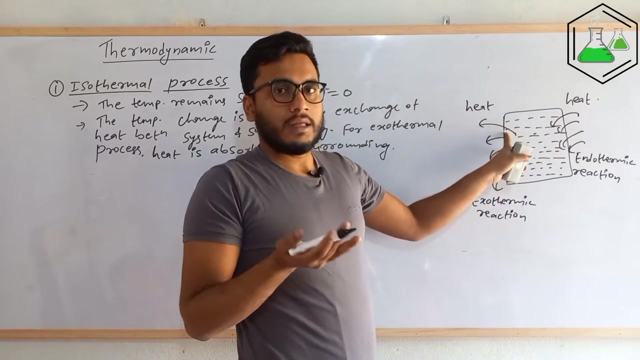 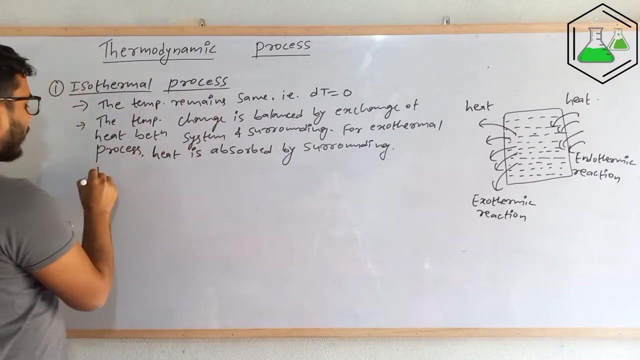 for the exothermal process, heat is absorbed by surrounding. it is absorbed by surrounding because in toward thermal process the temperature increases and that heat energy fino react. heat energy is absorbed by the surrounding to keep the temperature constant. similarly for endothermic process. for endothermic process, 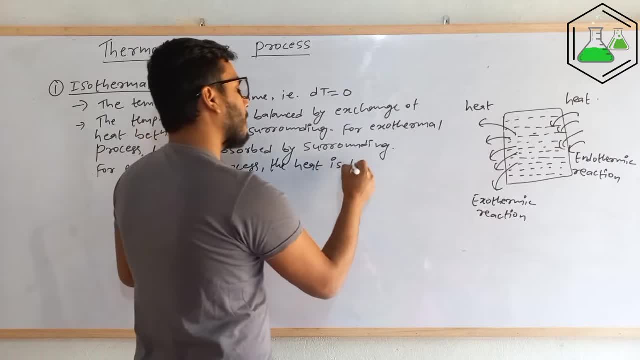 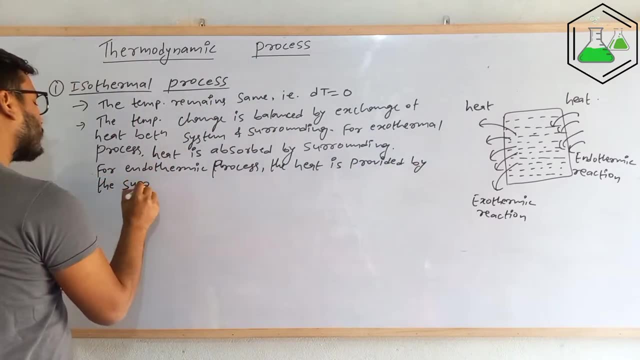 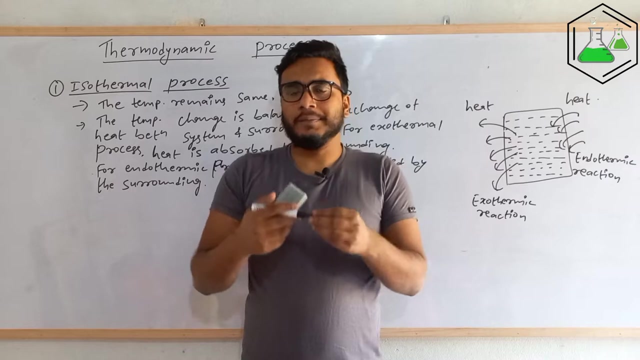 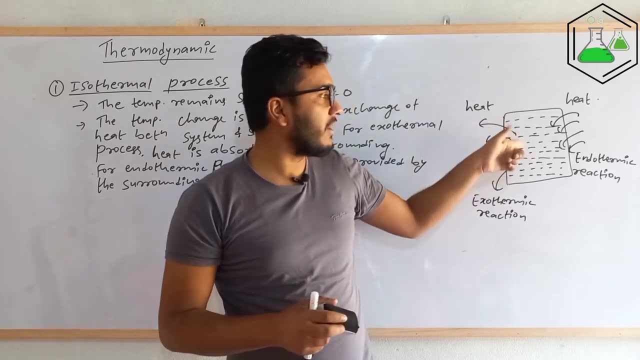 the heat is provided by the surrounding. by the surrounding, we know that in endothermic process, the temperature decreases and it needs energy in order to maintain the temperature, and that energy, or that heat energy, is provided by the surrounding, so that the temperature inside the thermostat will remain the same. now these 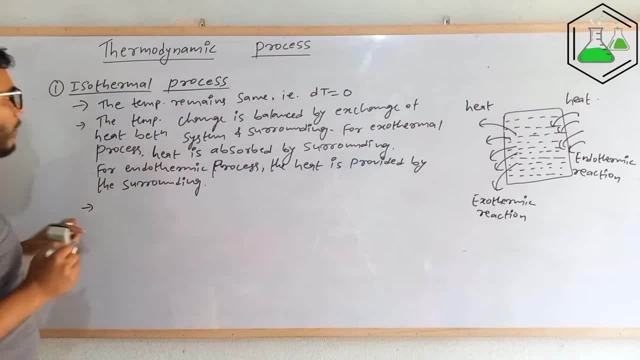 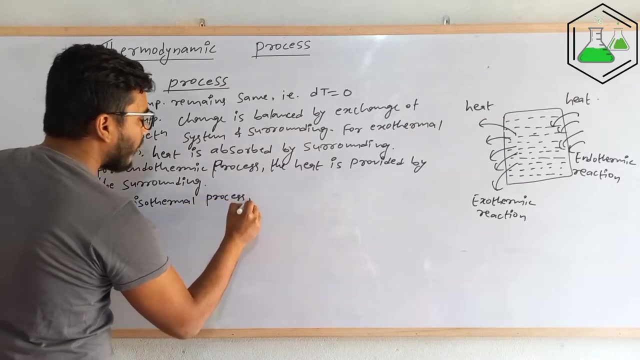 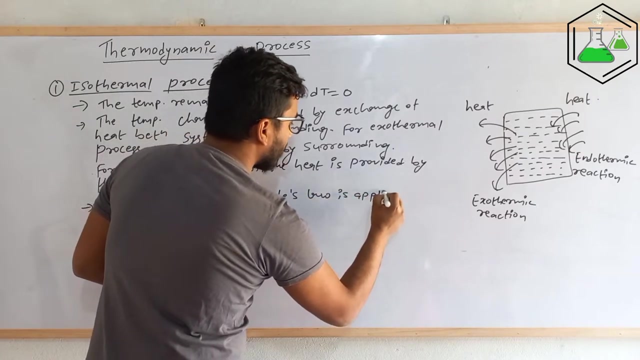 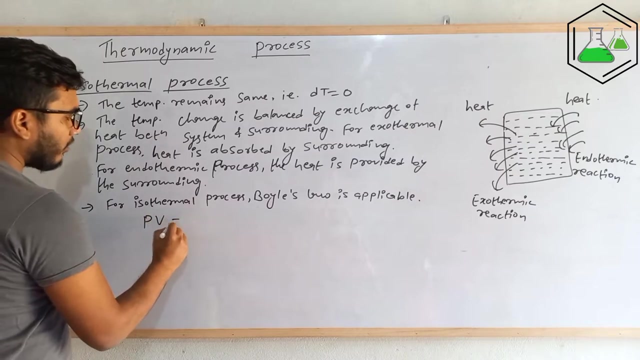 are the two points that you must remember now. another thing about isothermal process is that in isothermal process boyle's law can be applied. so for isothermal process, for isothermal process, boils law, boils law is applicable. applicable: the boils law states that the product of pressure and volume remains constant. in 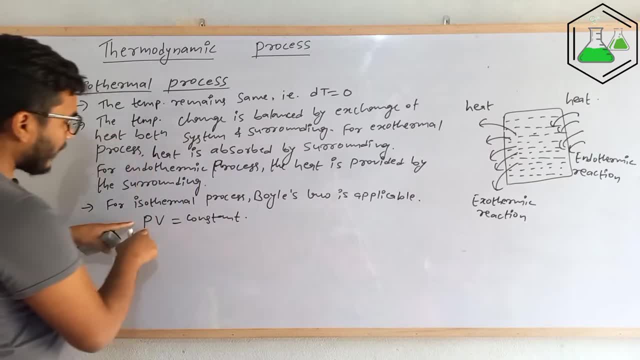 case of isothermal process. the product of pressure and volume of the system remains constant in case of isothermal process, so this can be written as: P 1 V 1 will be equal to P 2 V 2, and this is what we call the boils law. okay, these. 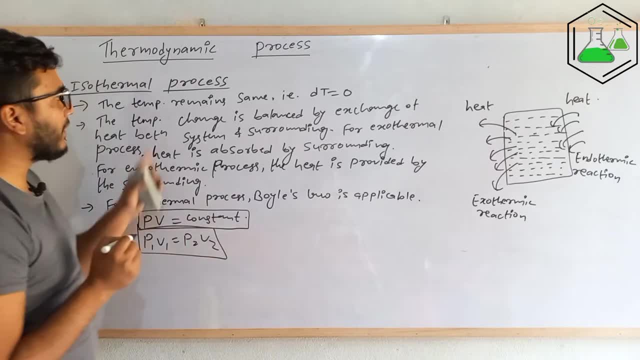 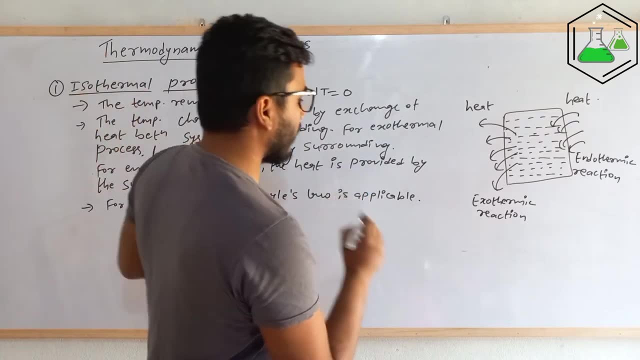 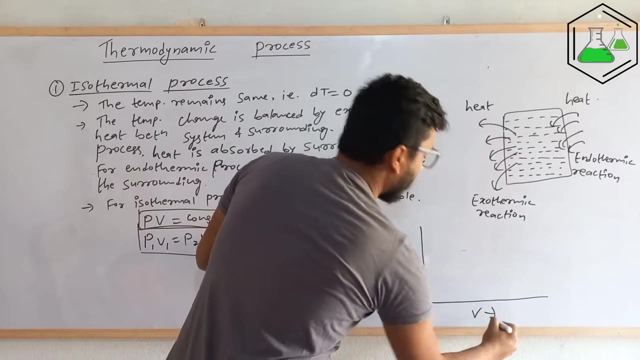 both are the boils law, and boils law is only applicable for isothermal process. now let's see how the process happens in graphical waveform. okay, let's make a graph over here. this is P and this is V, as the temperature is not changing, but pressure and volume might change. so if the pressure decreases, the volume 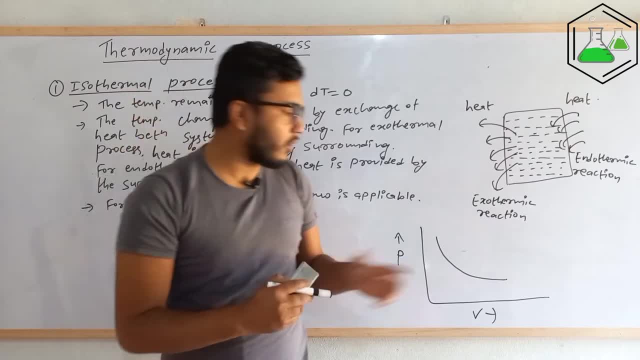 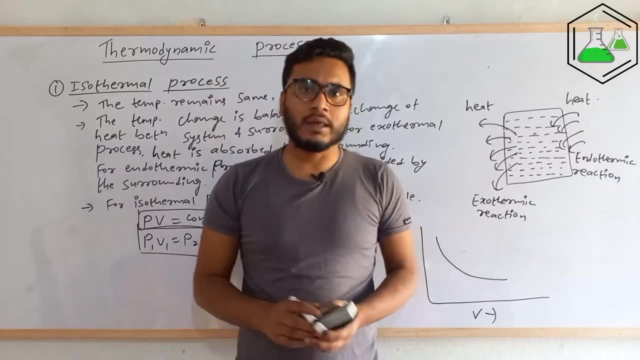 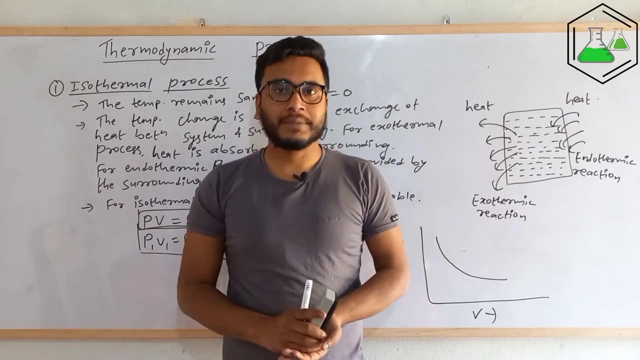 obviously will increase. so in isothermal process we get a curve like this if we plot pressure against volume. so this is what isothermal process actually is, in which the temperature should not change, but heat energy can be exchanged to balance the temperature. now let's see another process, that is, isobaric process. 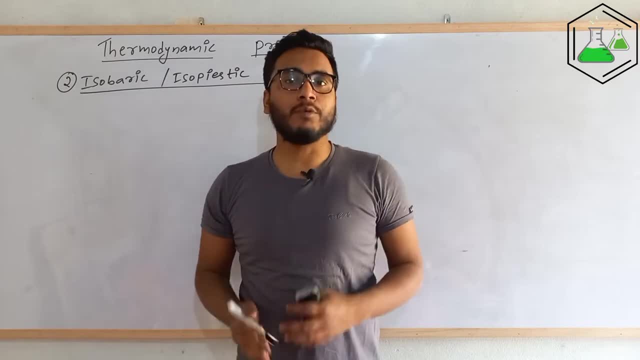 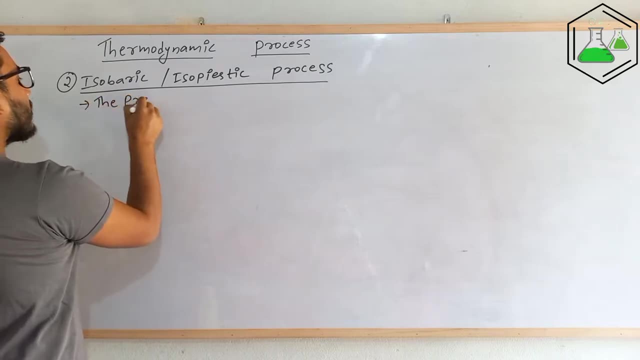 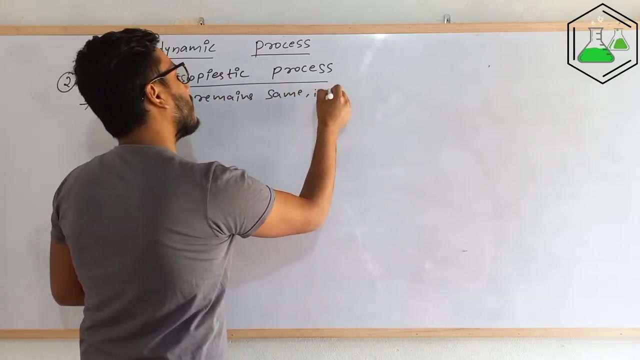 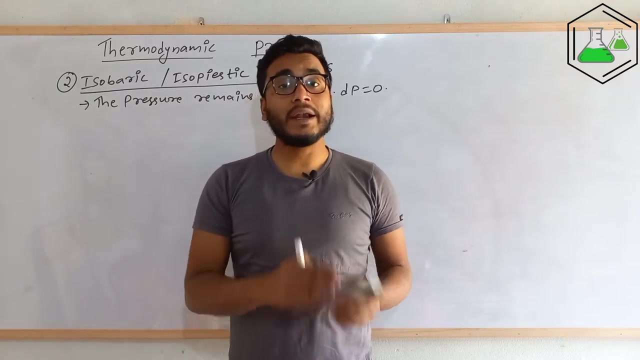 in isobaric process or isopistic process, the pressure in the system remains constant. let me write that the pressure, the pressure remains same, that is, DP will be equal to zero. now this type of process happens in a cylinder having weightless and frictionless piston. let us consider a cylinder in which the 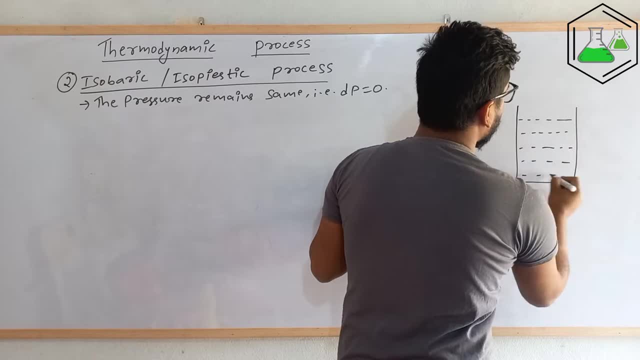 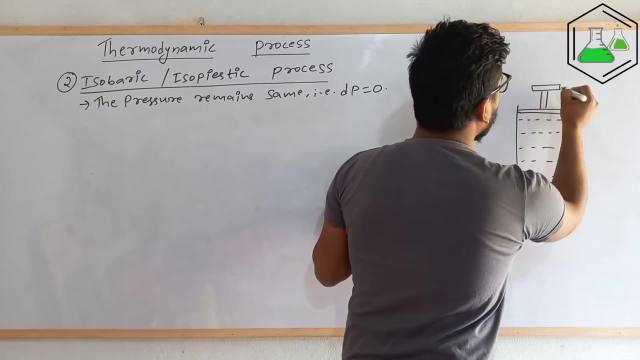 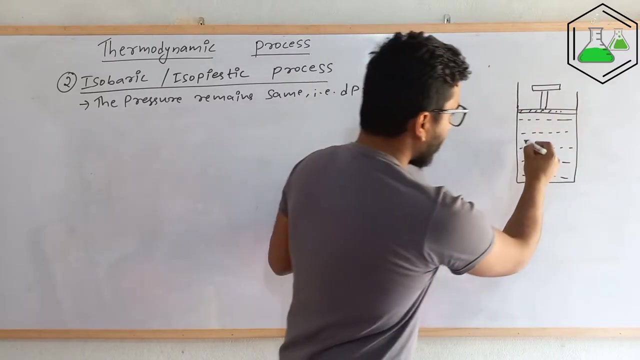 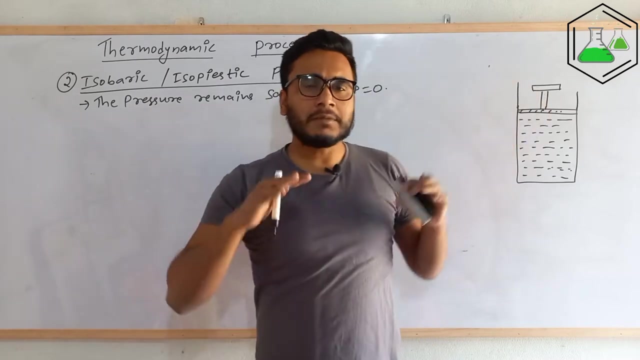 weight of this piston is under the bloody C and in this case, there is a substance under study and there is this weightless and frictionless piston. this is the weightless and frictionless piston. this can move up and down easily. okay, now, in this process, the pressure remains constant. okay, so this piston. 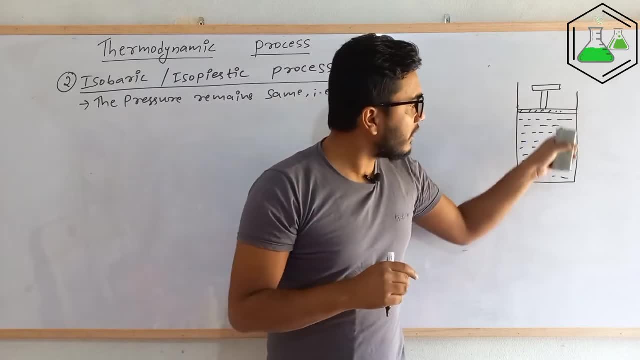 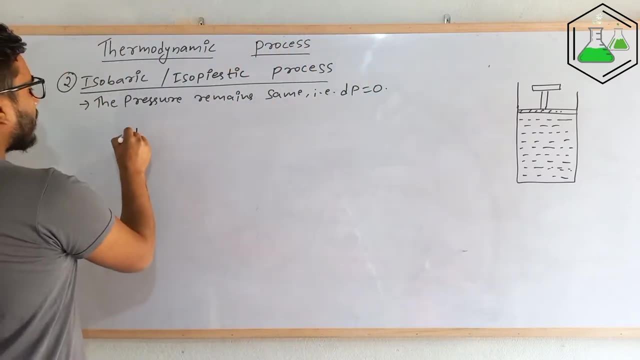 sometimes moves up, sometimes moves down in order to maintain the pressure. that on the change in volume of the system got confused. let me clear that. let us take an example of hydrogen and chlorine gas reacting with each other. so when hydrogen and chlorine are reacting, suppose in the cylinder there is 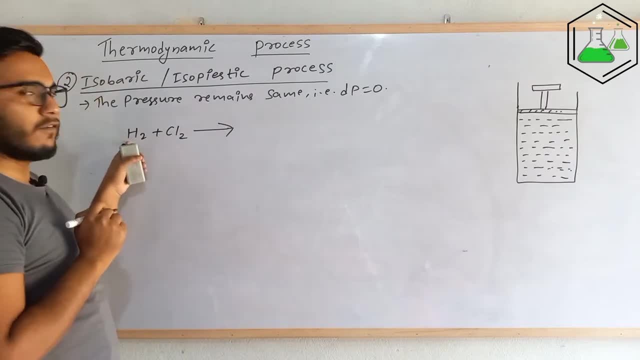 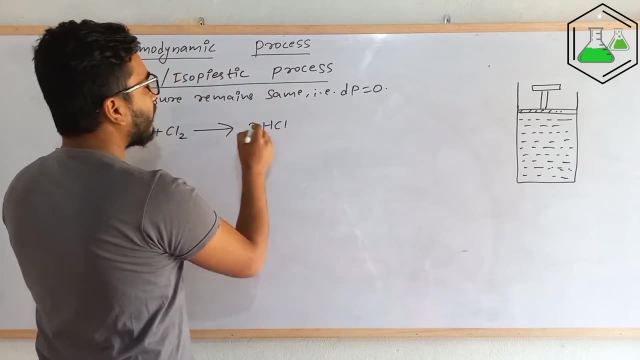 hydrogen and chlorine in one is to one ratio. so one mole of hydrogen, one mole of chlorine, and if they react they will form two mole of HCl. yeah, they will form two mole of HCl. so there are total two mole of reactant and two mole of product. 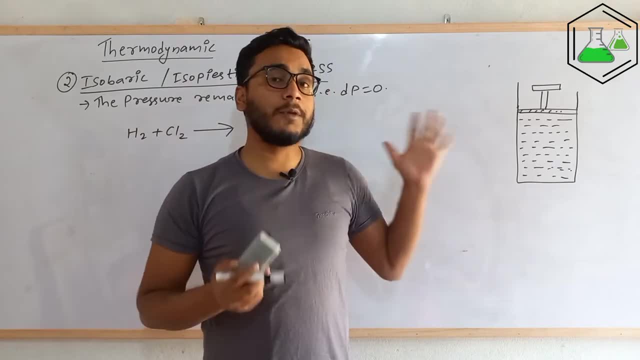 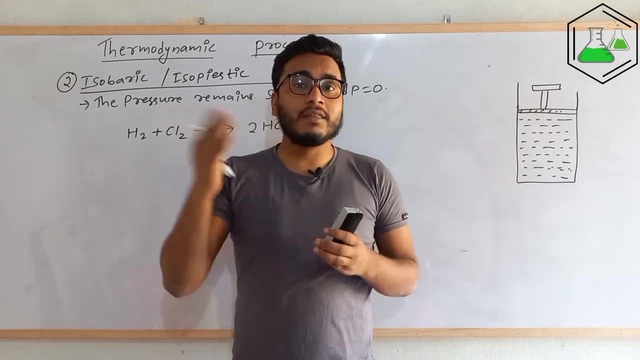 so will the volume change? no, the volume will not change. so in this particular case the piston will not move as the pressure is not changing, because we know that if volume changes, then only the pressure changes. if the volume do not change them, the pressure will not change and this process will easily happen. 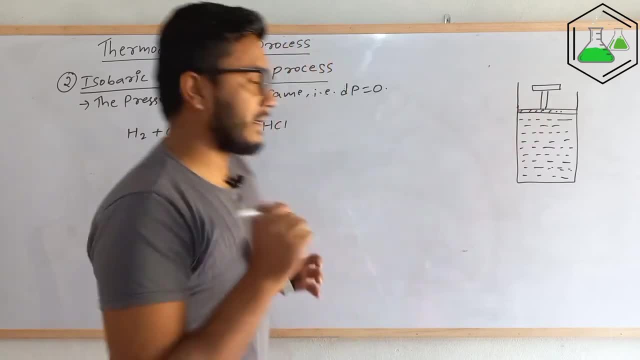 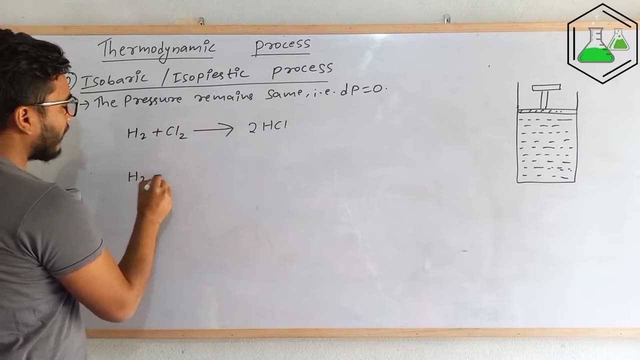 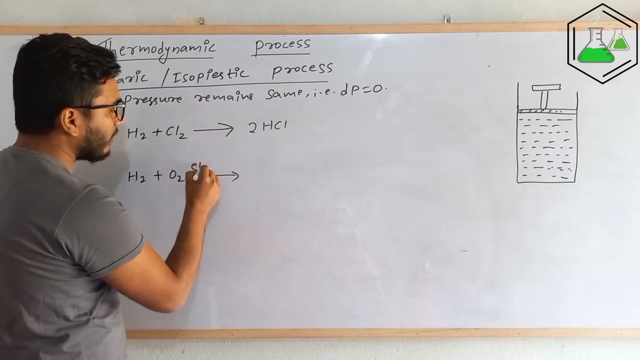 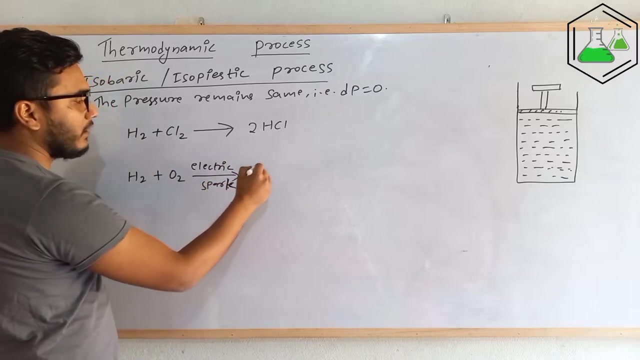 without the piston moving up or down. but what if we have? we take another reaction. that means there is hydrogen and oxygen. okay, there is hydrogen and oxygen in the cylinder and we provide electric spark to that electric spark we provide, we provide electric spark. then what will happen? it will form H2O, that is, water molecule. right to balance we have to put. 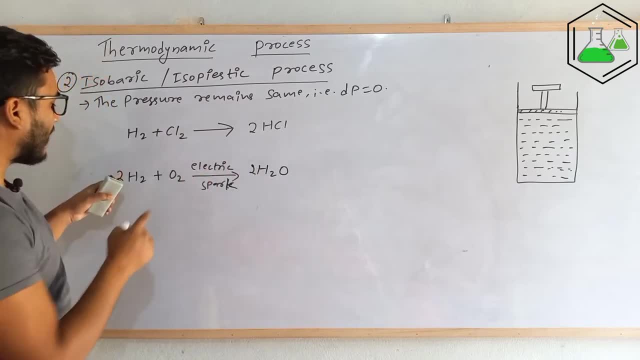 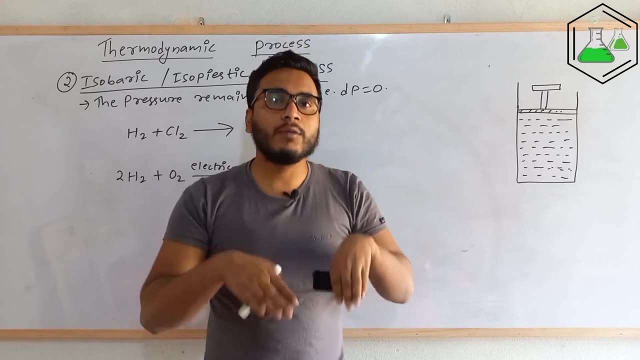 two over here and two over here. what do we see from here is that two plus one, three mole of reactant is forming only two mole of product. so in terms of its concentration, what will happen is the volume of blatant heraus germination increase, and this pulling of legislation should be. 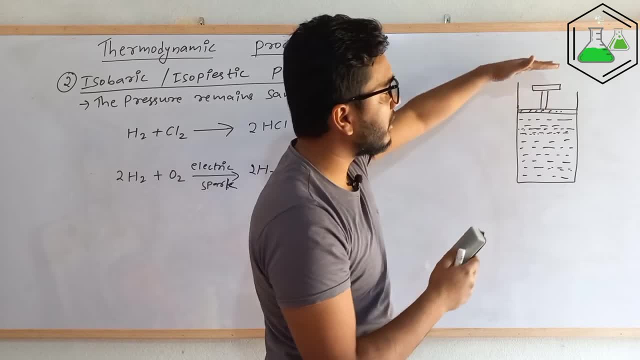 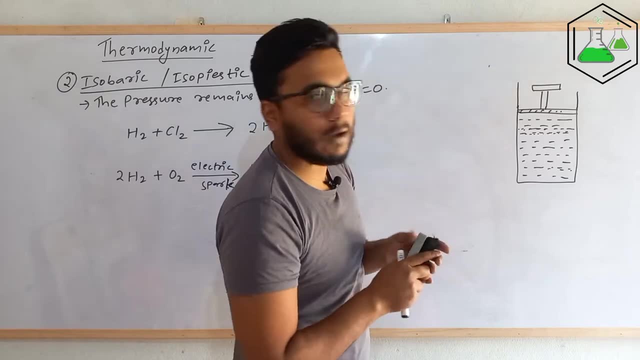 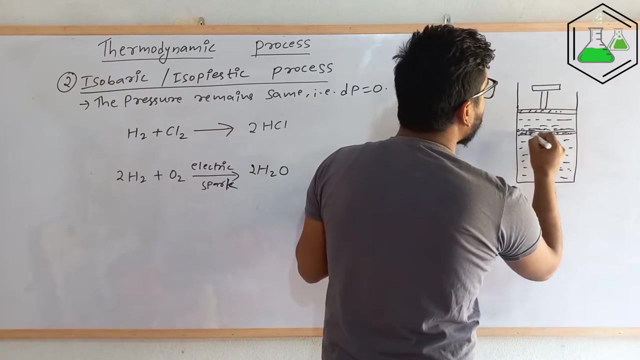 ART Luci by C and we will do that. so the pressure will decrease by twice, because three times the rê거든요 in relation to volume decrease. so output is the pressure. so if, if we just put this value, we get this value, if we just apply this value and we 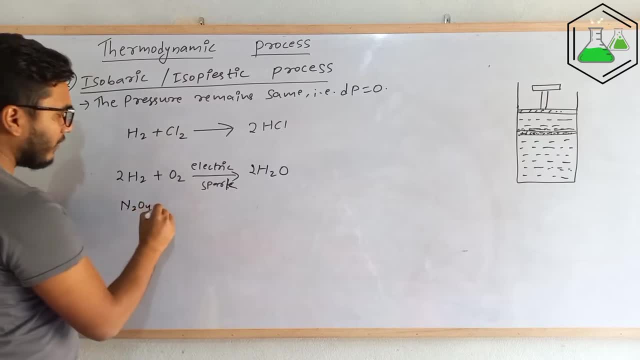 learn a tooth check based on this recipe? we can. the pressure for the piston is is dinitrogen tetroxide is giving nitrogen dioxide and if we react we get this. so one mole of dinitrogen tetroxide gives two mole of nitrogen dioxide. then 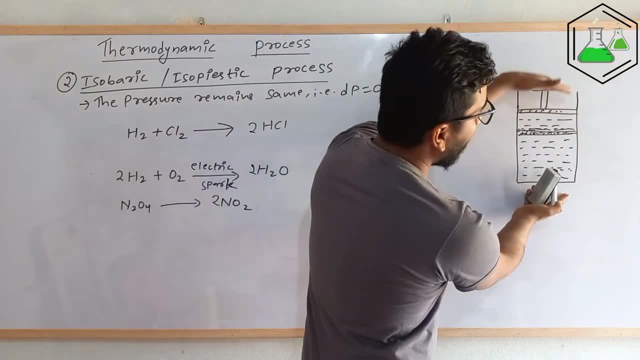 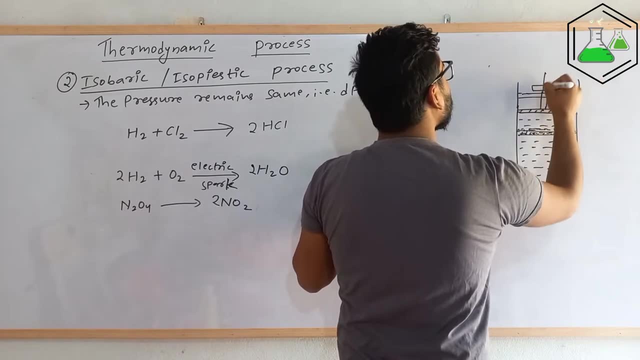 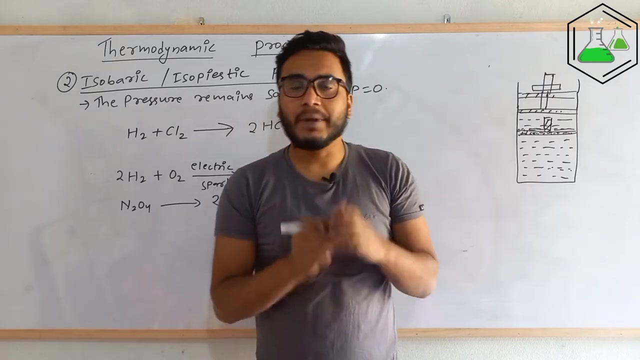 what happens? the volume is increasing. now this volume will increase, right? so in order to maintain the pressure, the piston moves up. the push piston now moves up. did you understand what I'm what I just said? to maintain the pressure equal, the piston sometime moves up, sometime moves down if the volume inside. 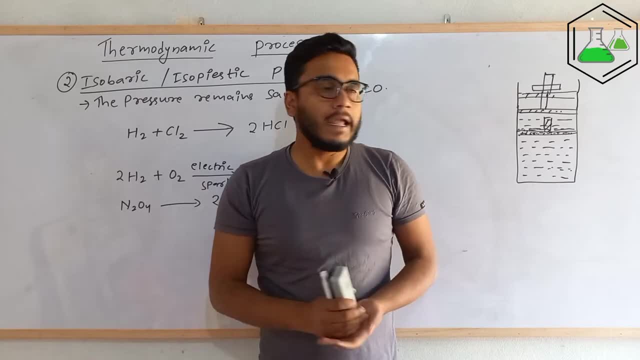 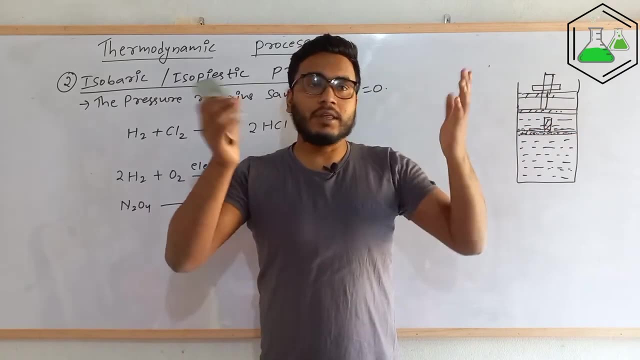 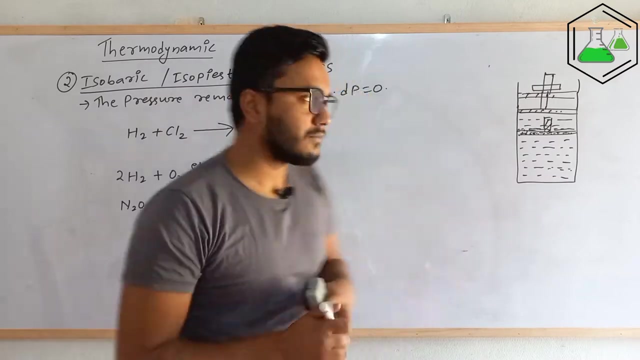 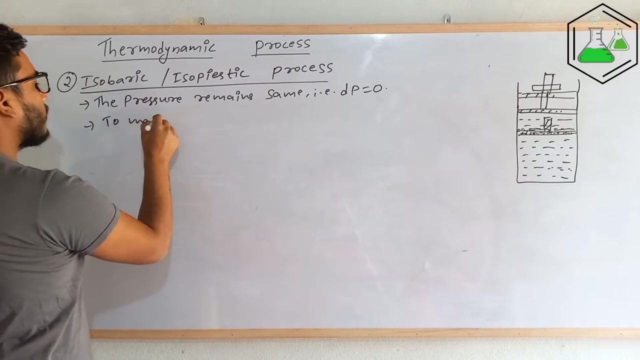 the system remains same, then the piston will not move. and if the volume inside the system decreases, the piston comes down. and if the volume inside the piston increases, then the piston will go up. and this is all for maintaining equal pressure. okay, so let me write it. to maintain: to maintain constant pressure. to maintain: 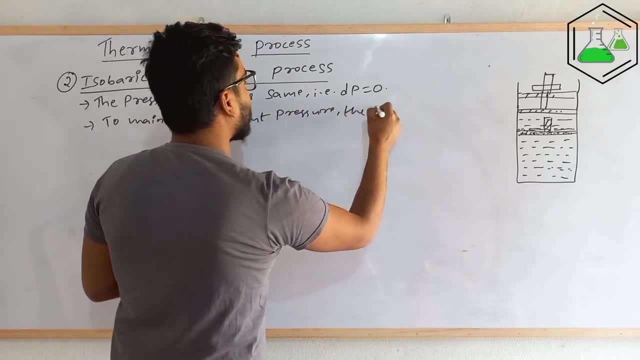 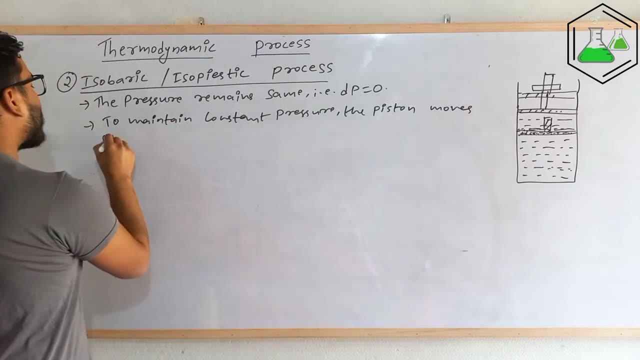 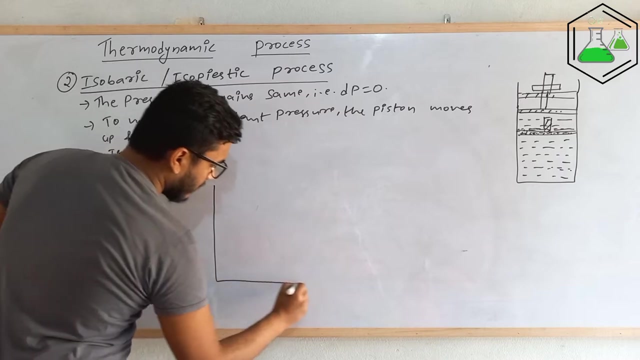 constant pressure, the piston. the piston moves, moves up and down, down. okay, now, similarly in third step in graphical form. similarly in third step in graphical form in graph, the isobaric process. or I to, in graphical form, the isobaric process. or I to, in graphical form, the isobaric process. or I to isopistic piece process. if we plot: 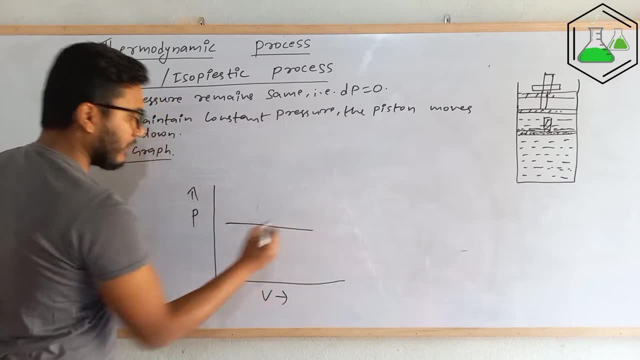 isopistic piece process. if we plot isopistic piece process, if we plot pressure against volume, then it will show pressure against volume. then it will show pressure against volume. then it will show a graph like this: we know that the. a graph like this: we know that the 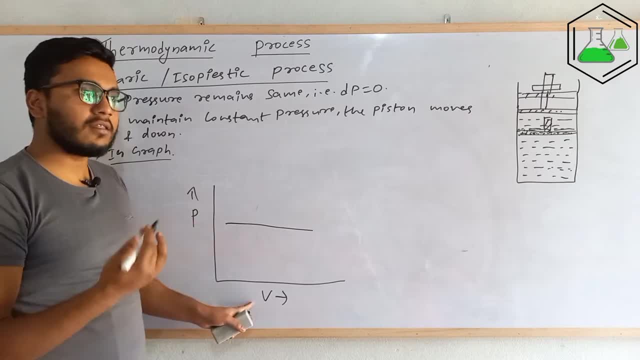 a graph like this, we know that the pressure will not change. even if the pressure will not change. even if the pressure will not change, even if the volume increases or decreases, the piston volume increases or decreases, the piston volume increases or decreases, the piston will balance that and the pressure will. 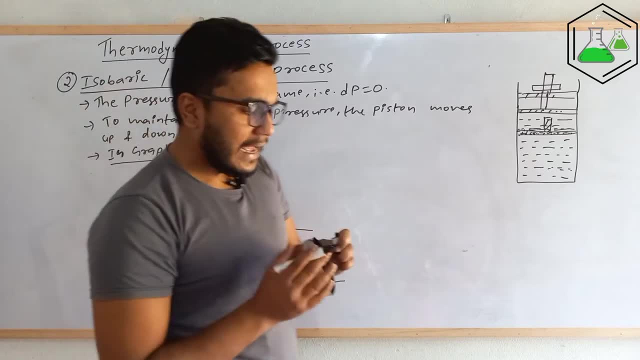 will balance that and the pressure will will balance that and the pressure will not change, and we get a graph like this: not change and we get a graph like this. So this is what isobaric or isopristic process actually is, in which the pressure remains. 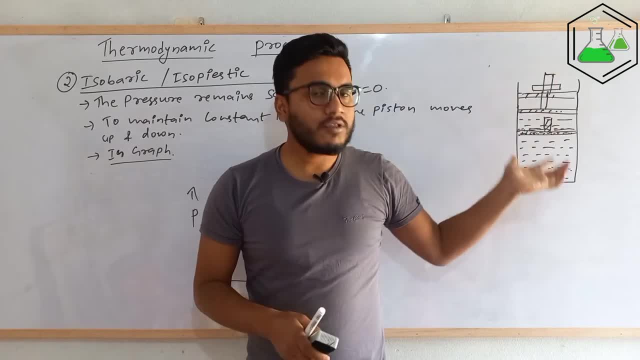 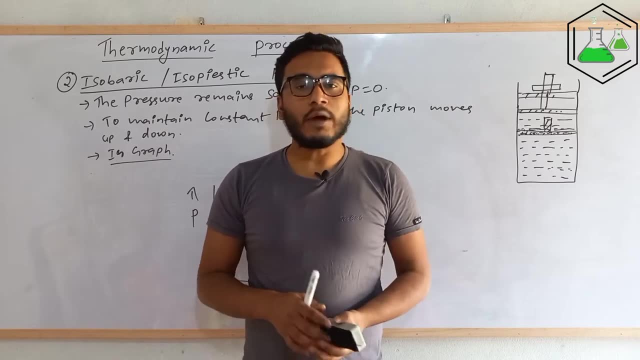 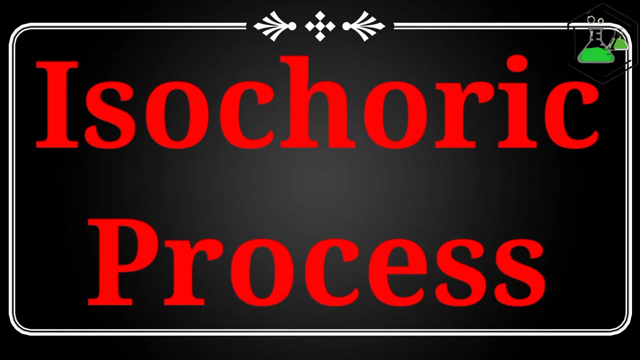 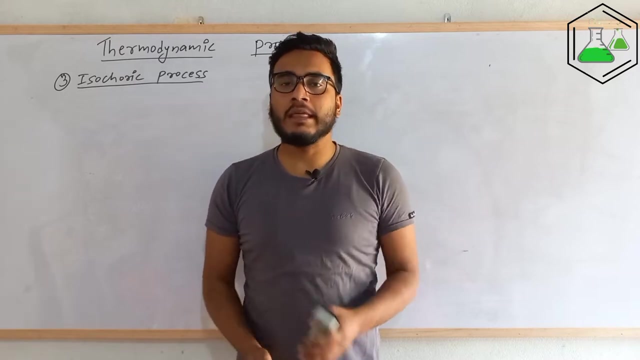 constant and to maintain the pressure the piston moves up and down, but the piston must be weightless and frictionless. that is the criteria. okay, So I hope you understood about isobaric process. Now let's understand the isochoric process. In isochoric process, the volume of the system remains same. Let me write that. 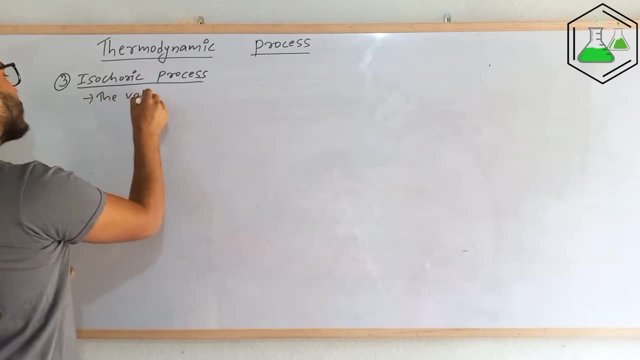 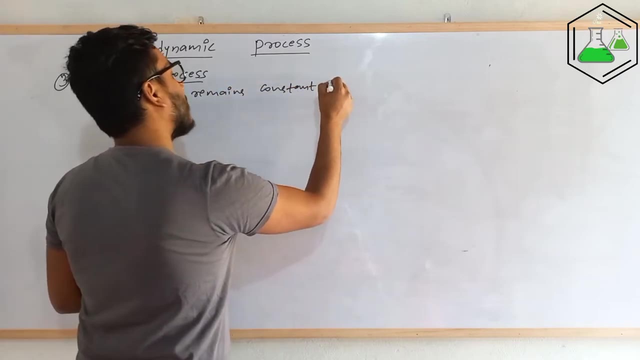 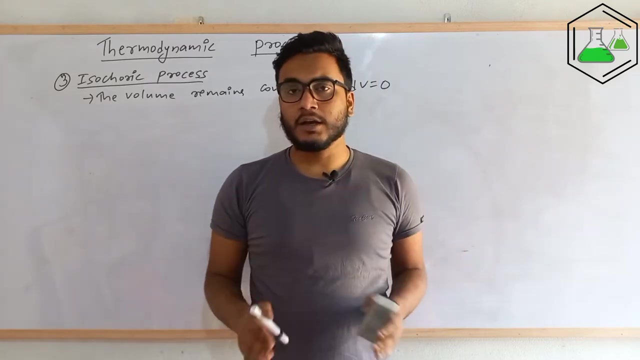 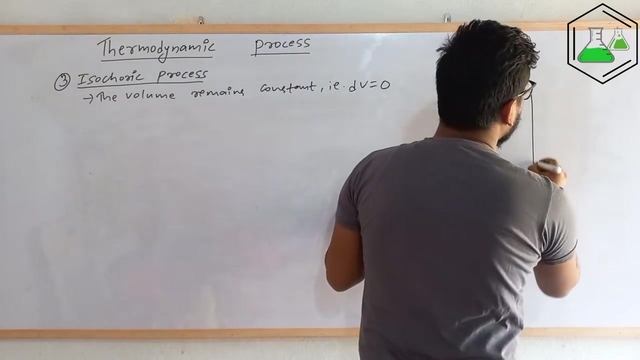 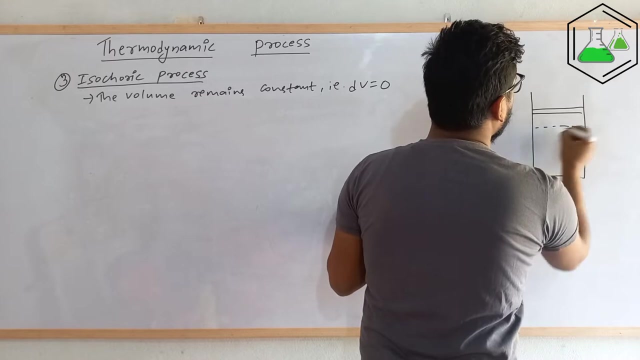 the volume remains constant. the volume remains constant, that is, dv will be equal to zero. and this type of process happens in a cylinder with fixed piston. The piston do not move up and down. So let us consider a system in which the substance is put over here. 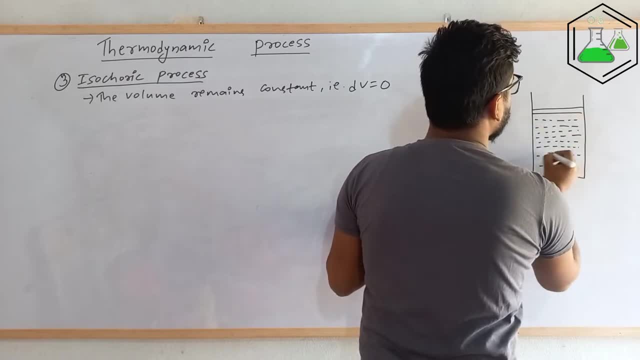 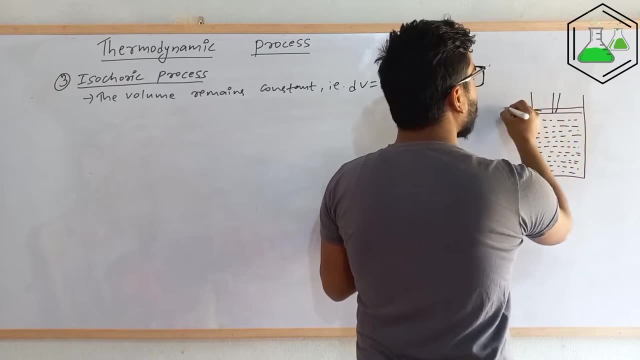 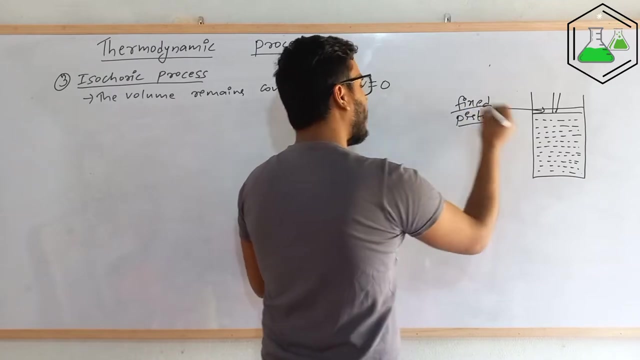 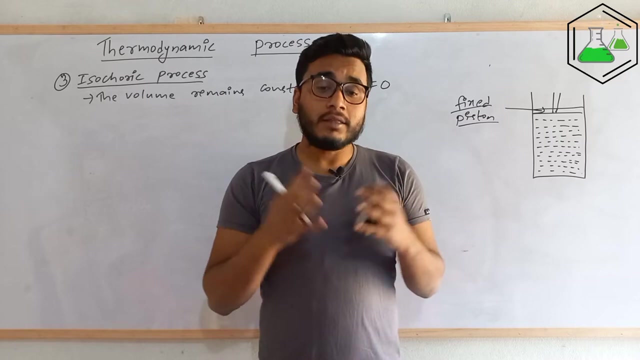 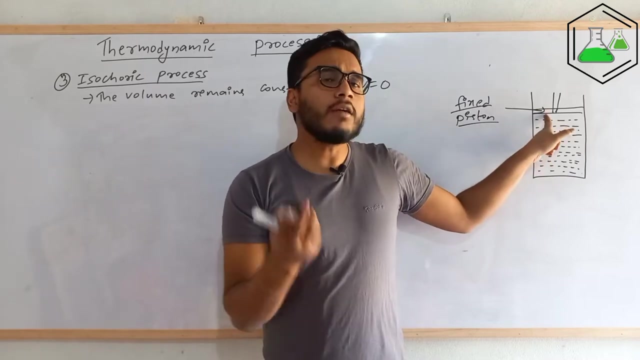 The substance is put over here and this piston is fixed. This is a fixed piston, that is, it will not go up, it will not come down. the reaction happens. suppose the reaction happens over here now. let us consider the volume increased. okay, let us consider the volume is increasing. now the piston is supposed to go up, but as it is fixed, it cannot go up. 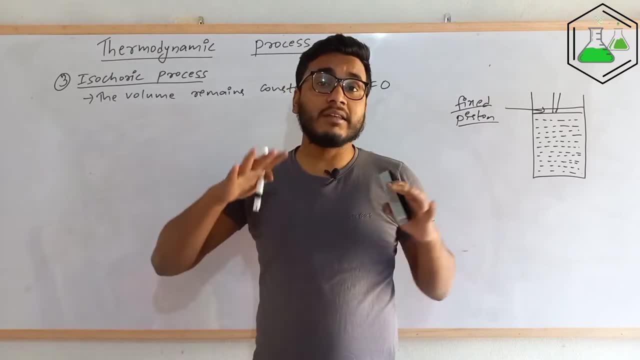 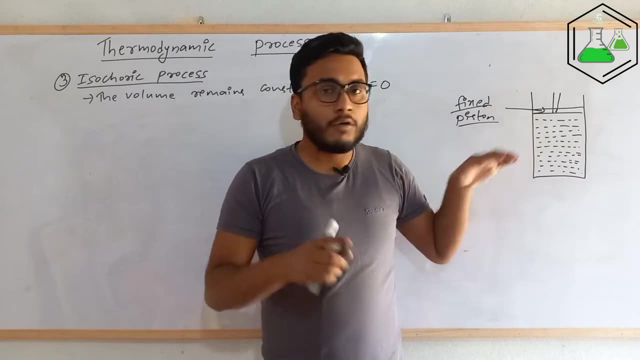 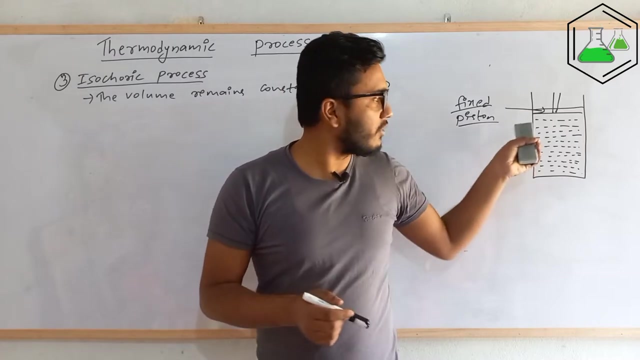 now, to maintain that equal volume, the pressure inside the system also increases, so that the volume would not go up. Similarly, in a reaction in which the volume is supposed to decrease, the pressure also also decreases, so that the volume will remain constant. So in this type of process fixed piston is used, that is, piston should not move at all. 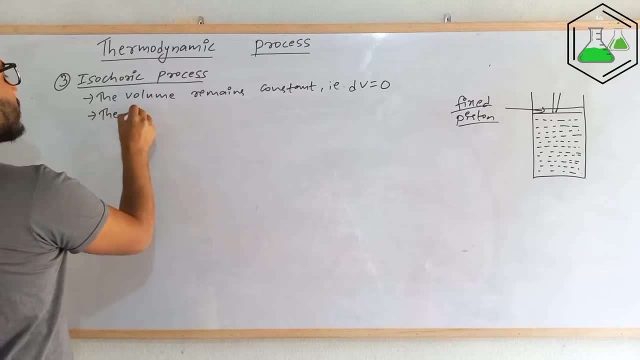 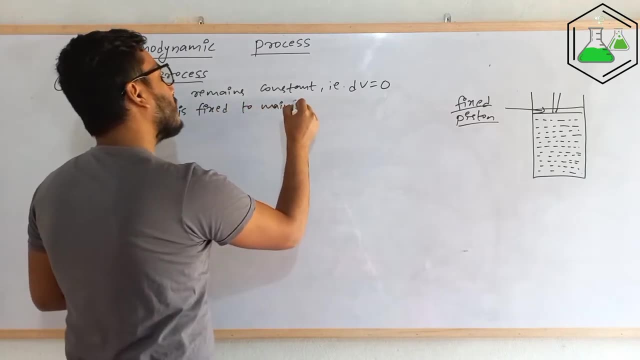 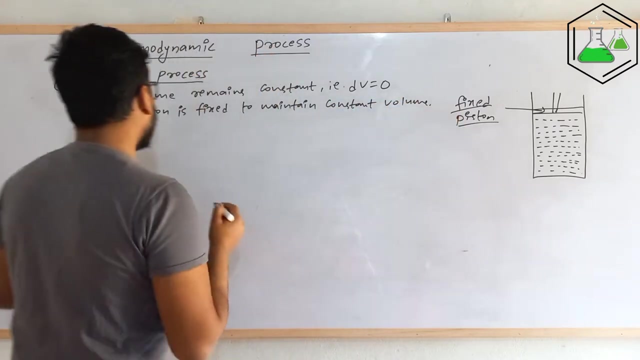 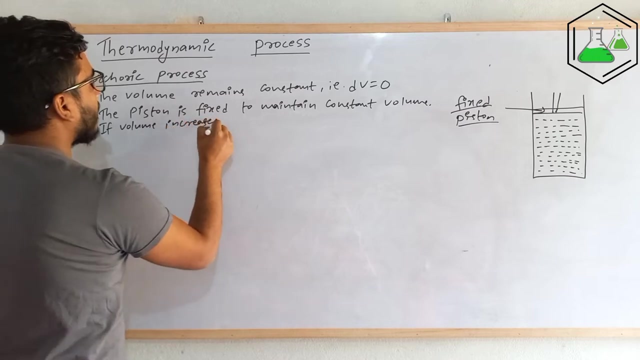 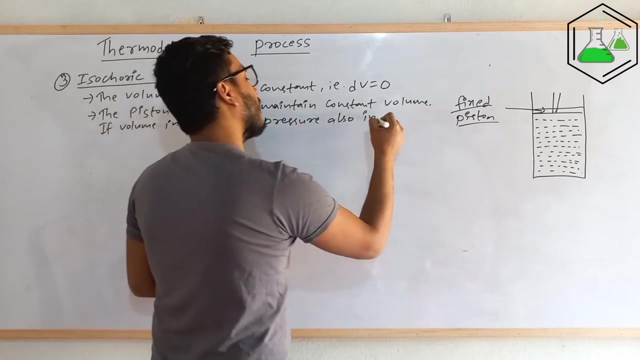 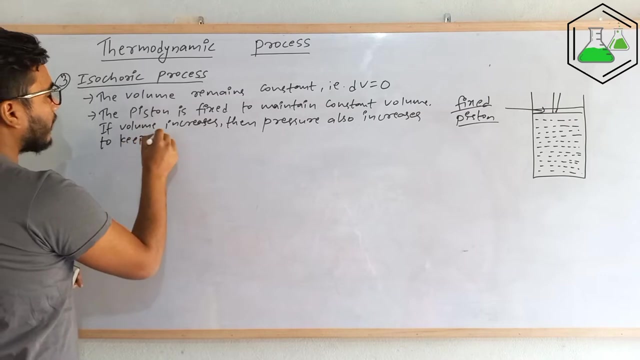 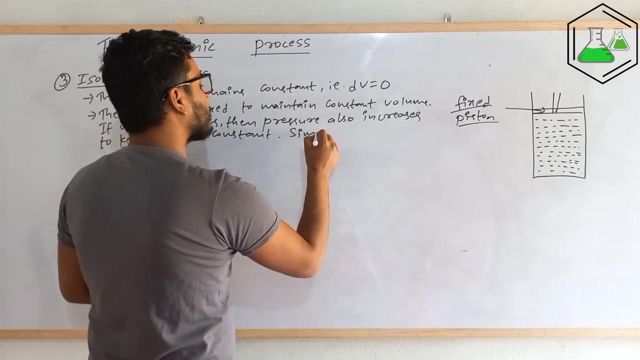 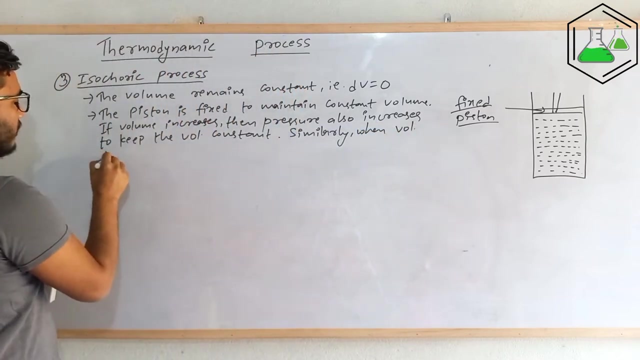 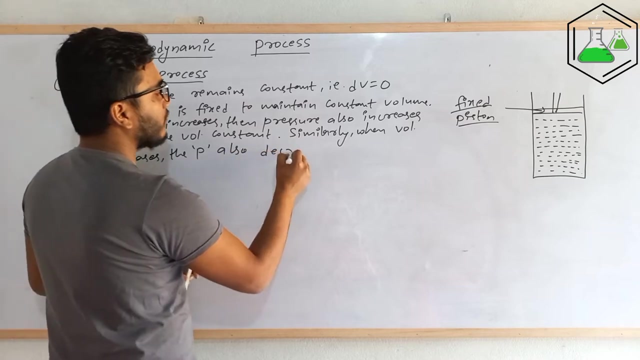 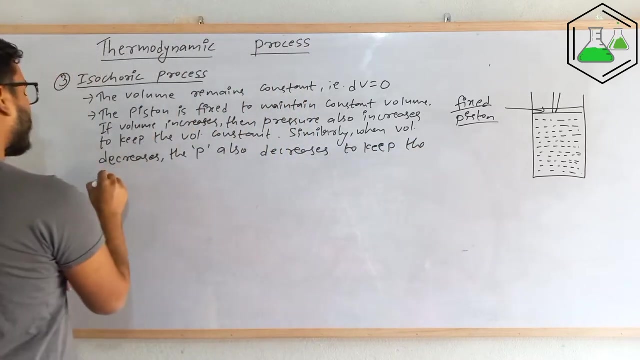 So the piston, the piston is fixed, fixed to maintain, to maintain, constant, to maintain volume, constant, volume. if volume increases, if volume increases, then pressure also increases, then pressure also increases to keep the volume constant, constant. similarly, similarly, when volume decreases, when volume decreases, the pressure also decreases to keep the volume constant. so 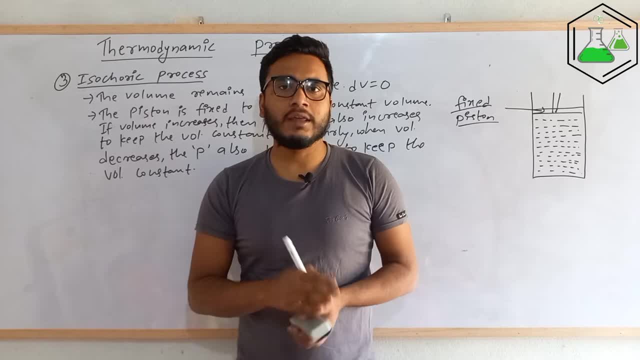 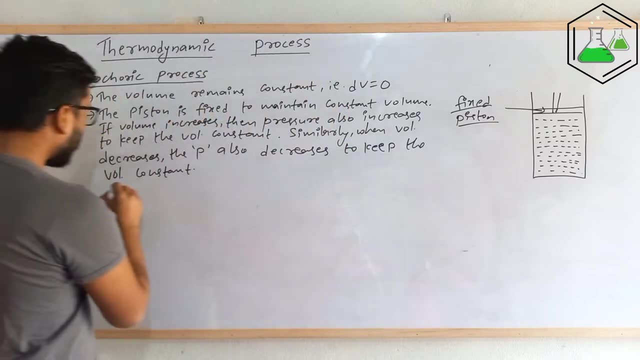 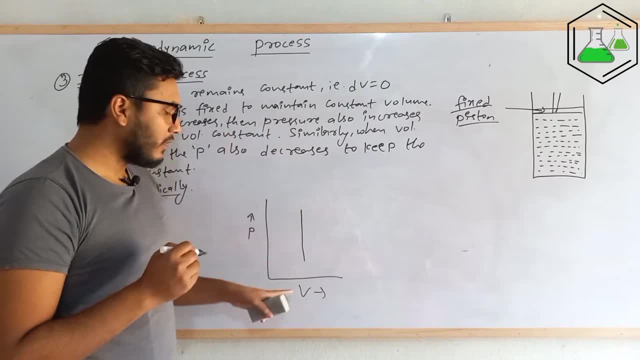 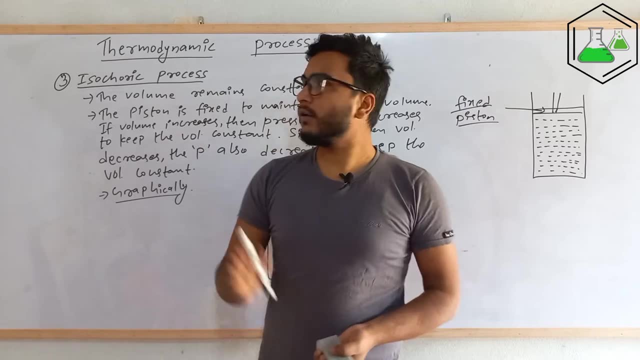 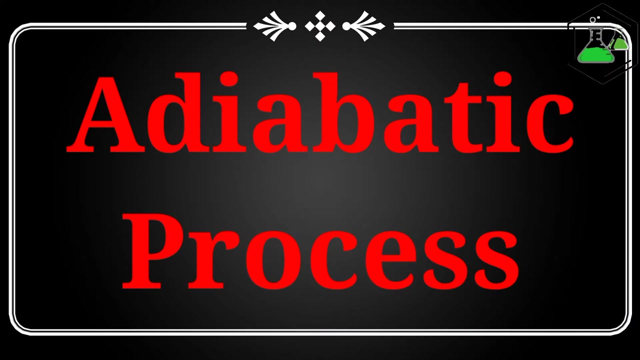 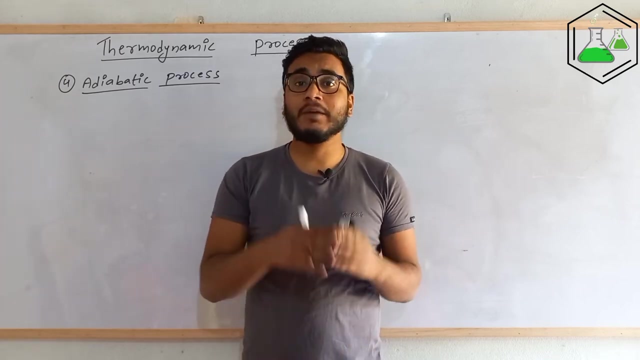 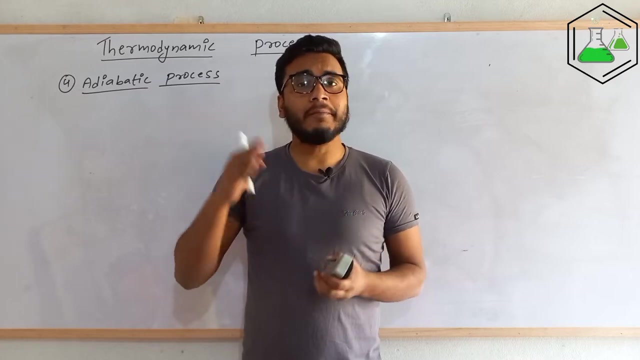 like this: even if the pressure increases or decreases, the volume will always remain the same, okay, okay, that's why a fixed piston is used over there. i hope you understood what isochoric process actually is. now let's see the adiabatic process. in adiabatic process, the boundary is adiabatic. that means the system and the surrounding is separated by an adiabatic wall that does not allow the heat and matter to exchange between them. 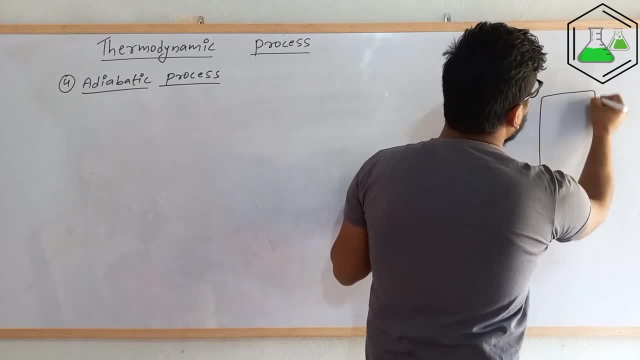 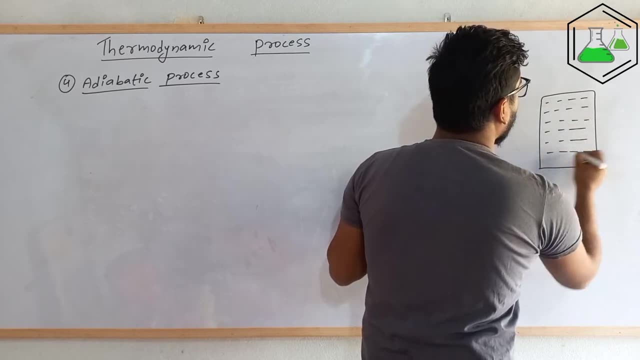 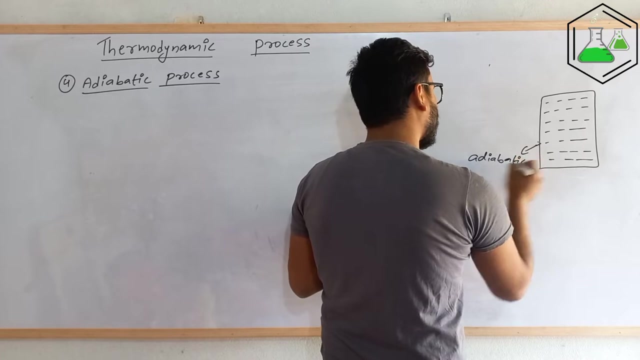 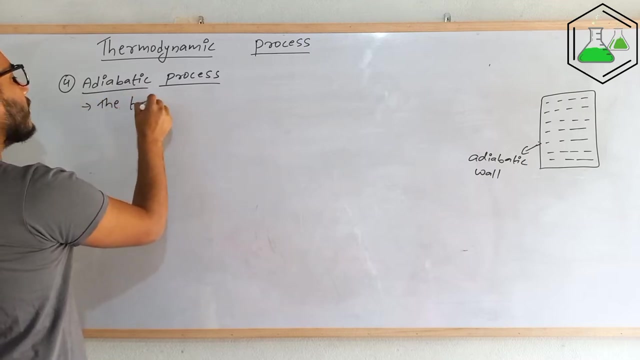 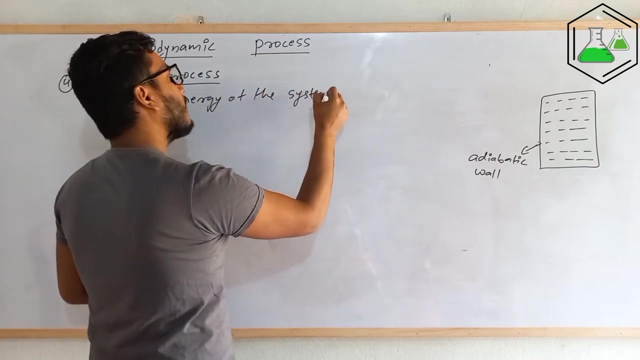 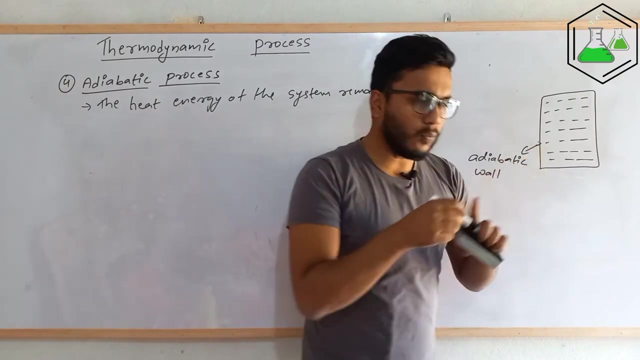 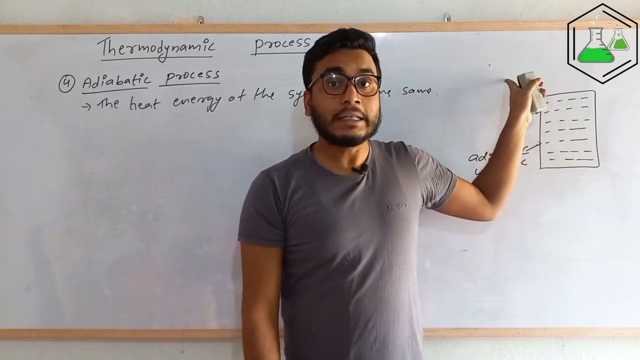 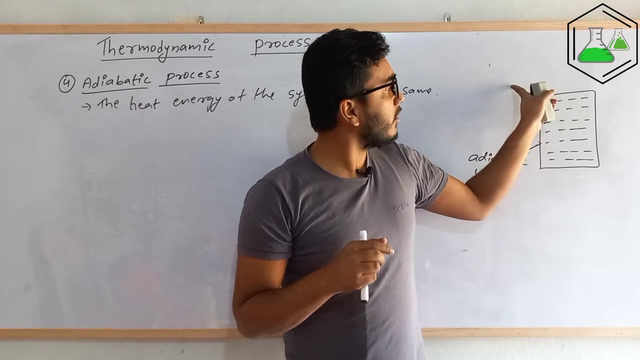 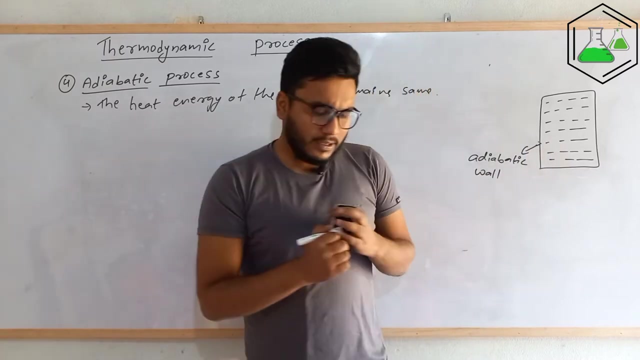 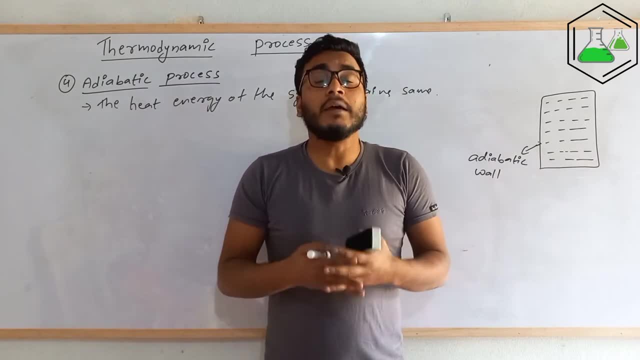 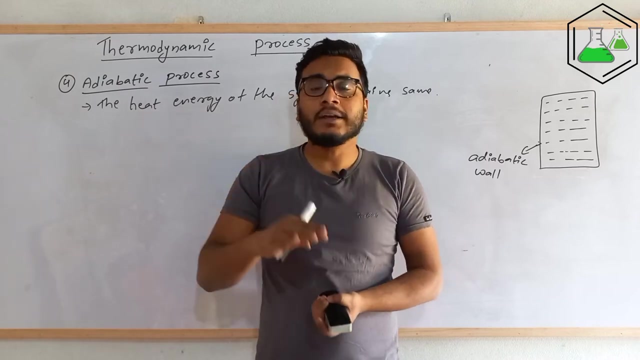 system. then what happens? in exothermic process there is very much heat, heat energy right now that needs to go out and that cannot go out. and to balance that heat energy, the temperature increases. okay, to balance that heat energy, to keep the heat energy of the system constant, the temperature. 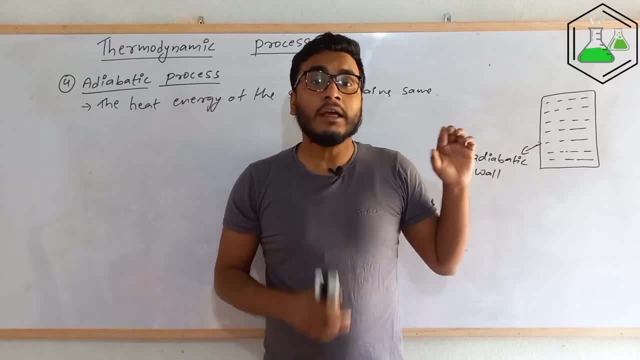 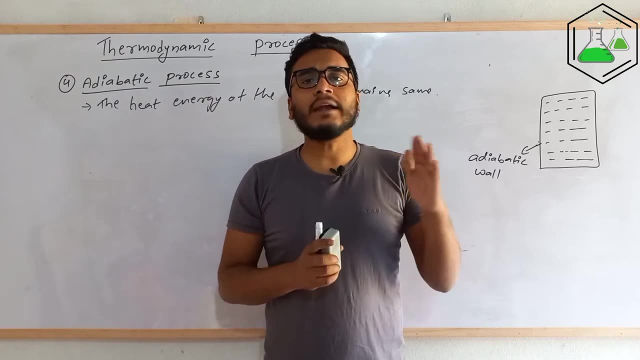 increases. similarly, in case of endothermic reaction, there should it should get heat energy right. so heat energy will decrease in case of endothermic reaction and to keep that heat energy constant, the temperature of the system decreases but it does not either take or give the heat. 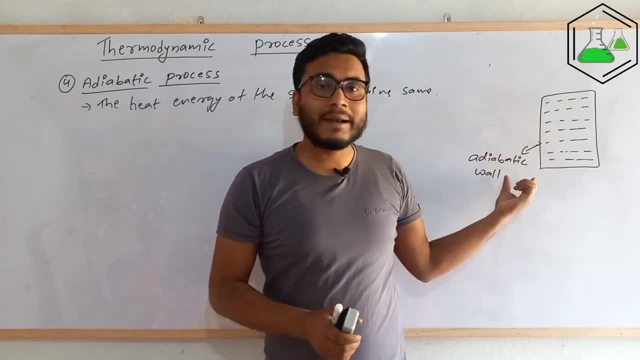 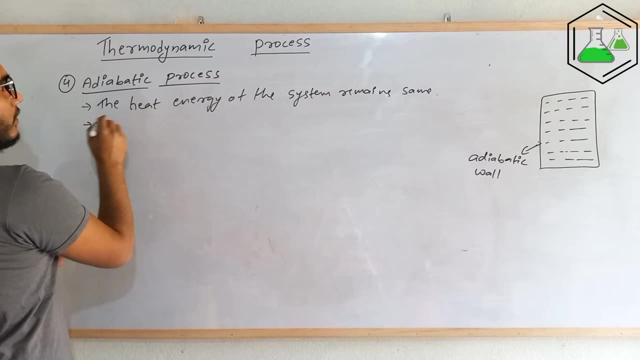 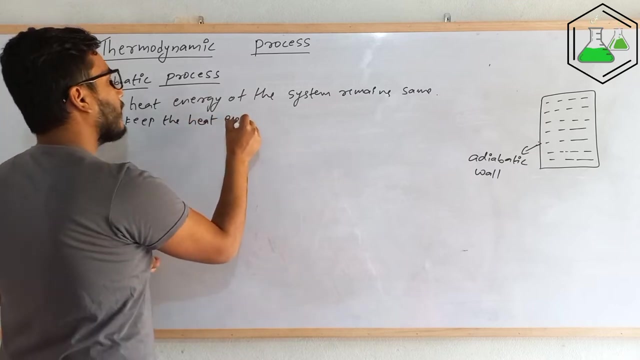 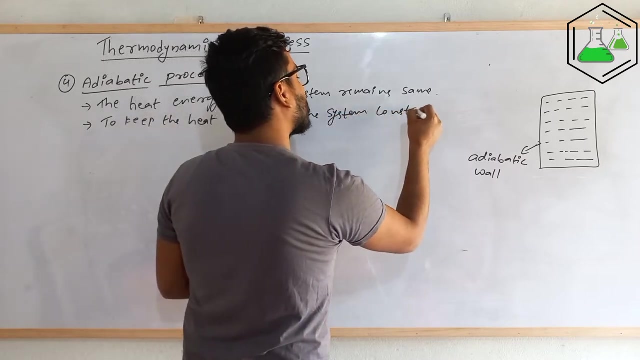 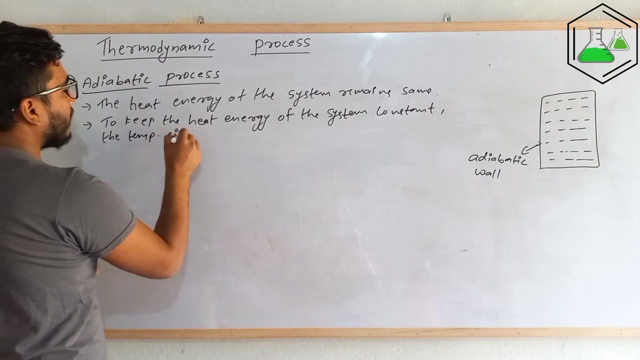 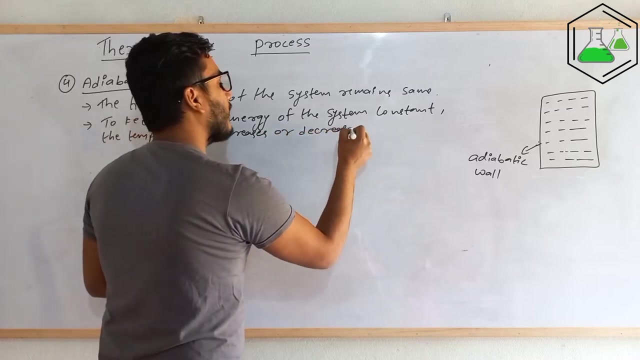 energy to the surrounding. that is, the work of adiabatic wall that does not allow it to do so. so let me write that: uh, to keep, to keep the heat energy of the system constant. constant the temperature. the temperature either increases or decreases in case of, in case of 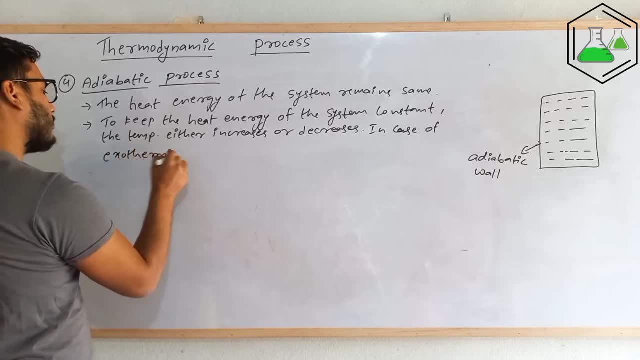 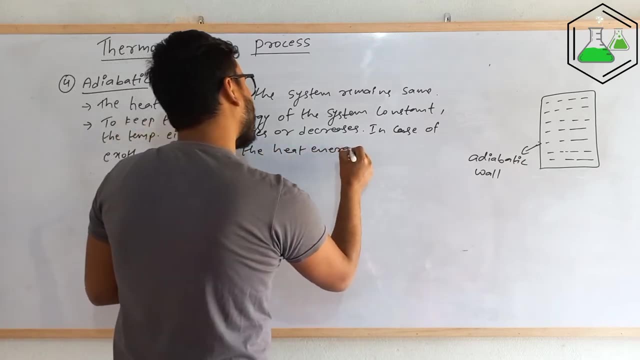 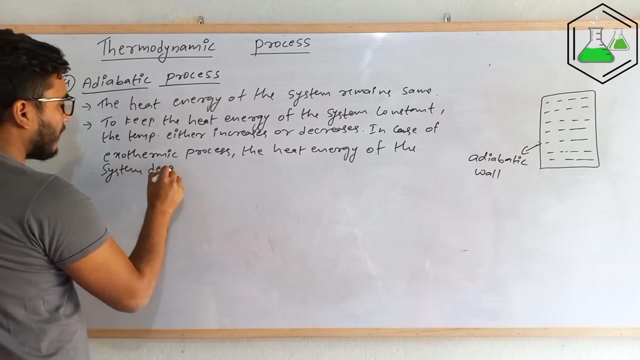 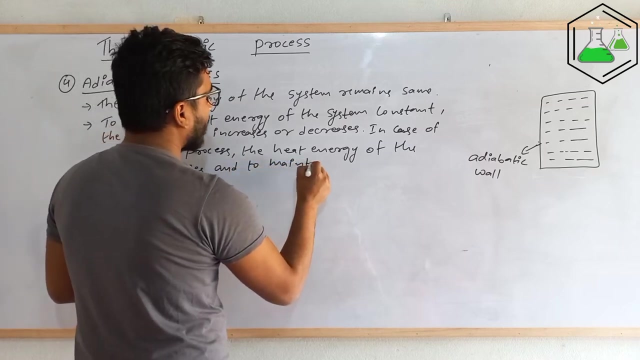 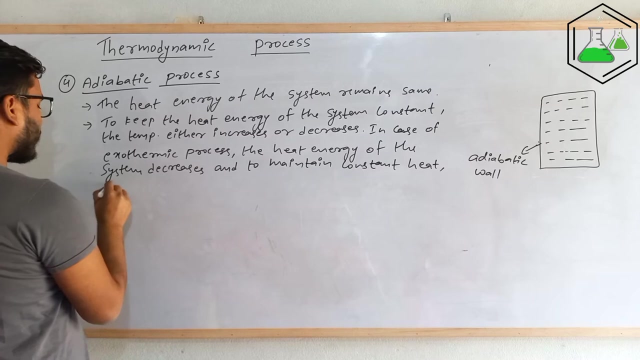 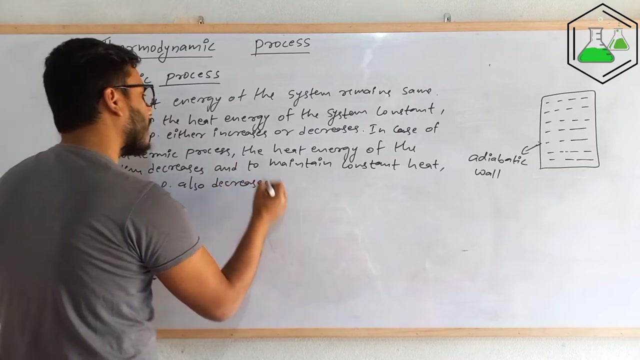 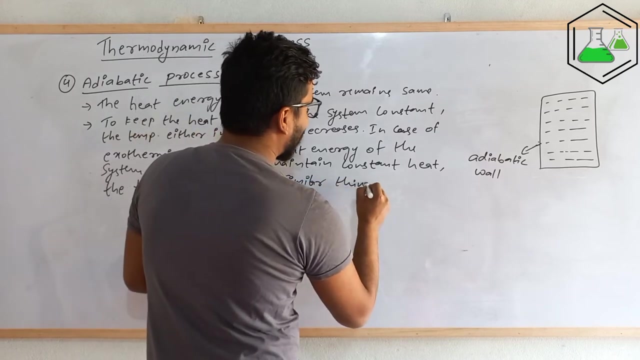 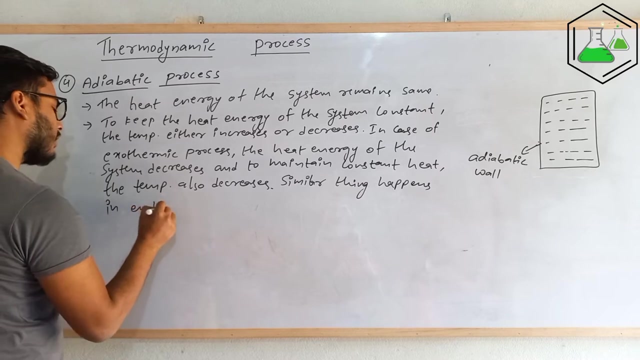 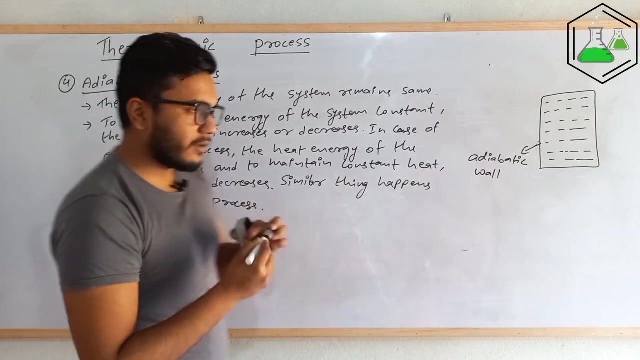 exothermic process, the heat energy. the heat energy of the system system decreases, decreases. and to maintain, to maintain constant heat, to maintain constant heat: the temperature. the temperature also decreases, the the temperature also decreases. similar, similar thing happens, happens in endothermic process, endothermic process. so in endothermic process, the heat energy of the system decreases and 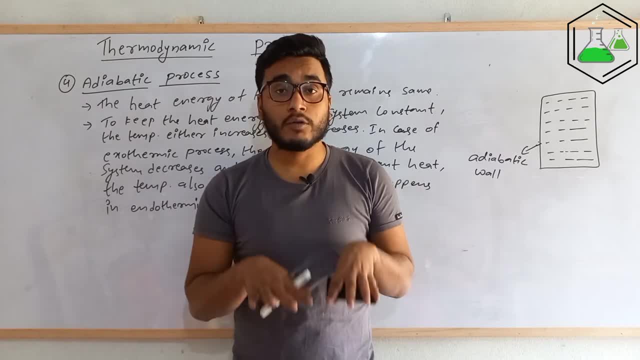 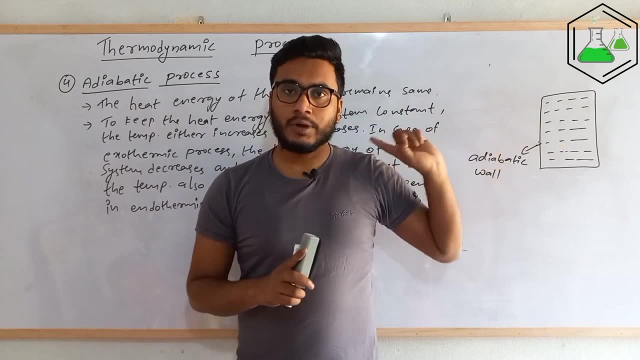 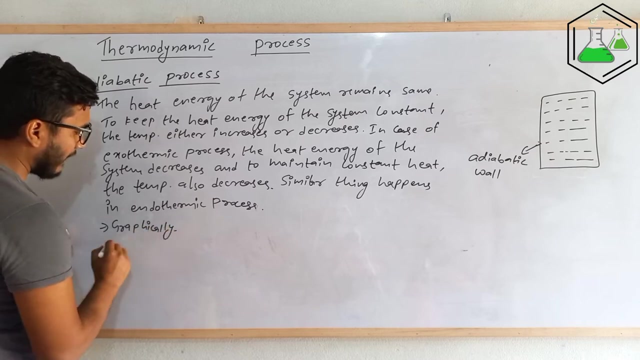 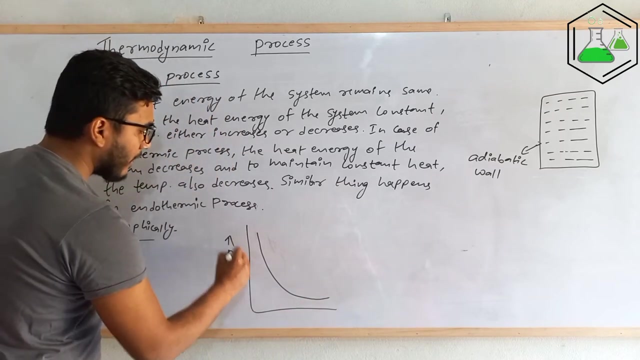 to maintain that heat energy constant, the temperature of the system also decreases, but there is no exchange of heat and matter between the system and the surrounding. okay, and graphically, if we see this process, then we get a graph like this. the graph is little bit similar to the isothermal process, but it is more steeper than the isothermal process. so for adiabatic, 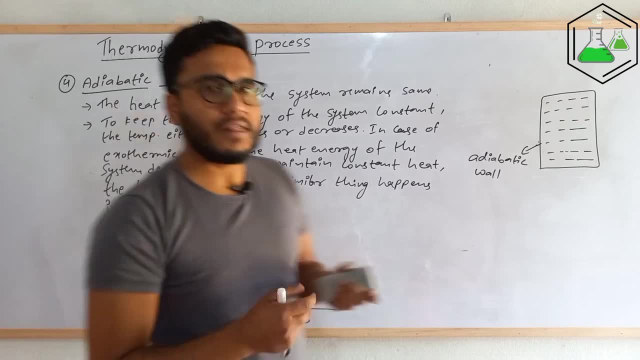 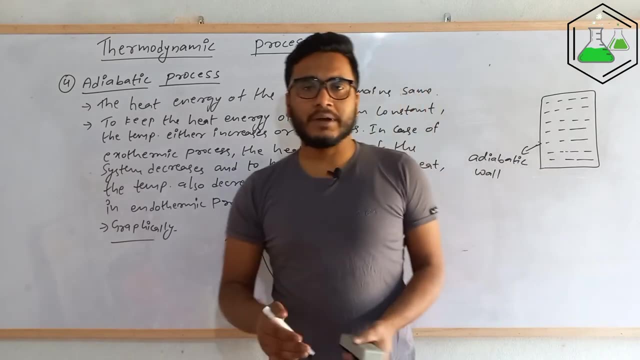 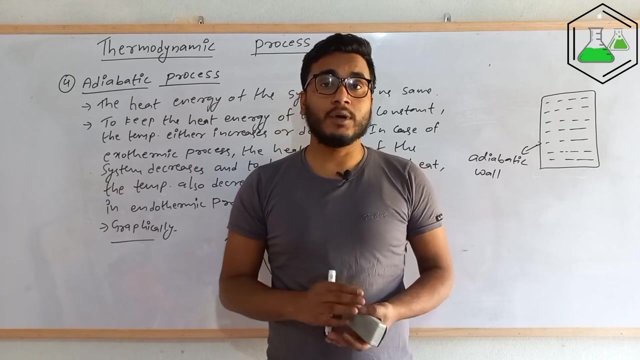 process. we get a graph like this, because pressure and volume will obviously decrease, but the temperature will obviously change, and we get similar type of graph as in the isothermal process, but this is more steeper than that one. i hope you understood everything about adiabatic process. now let's see the last one and one of the most important one, that is: 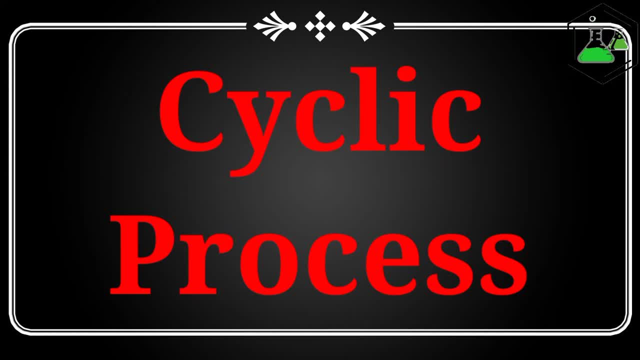 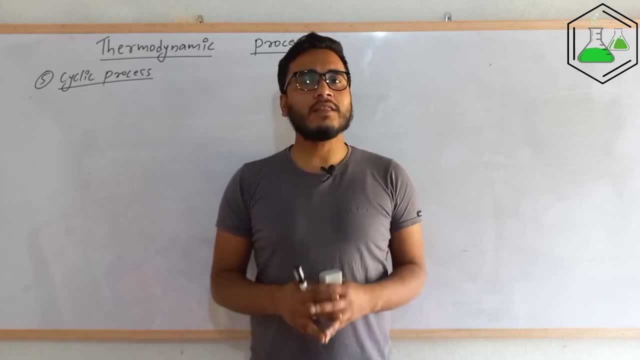 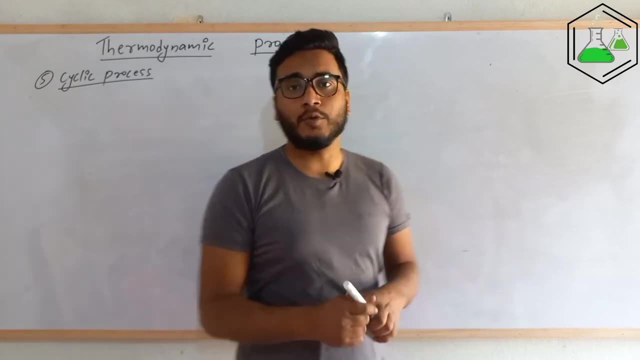 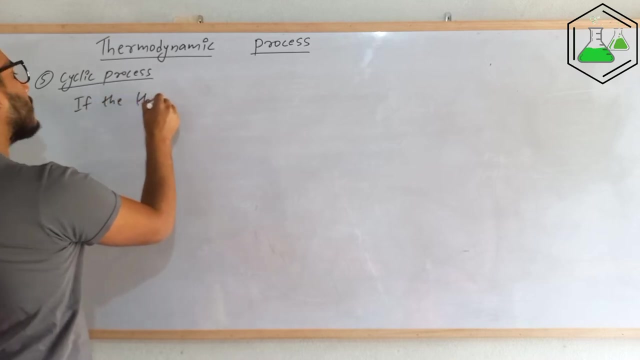 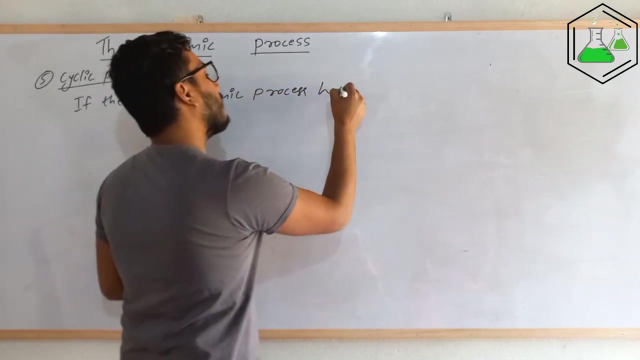 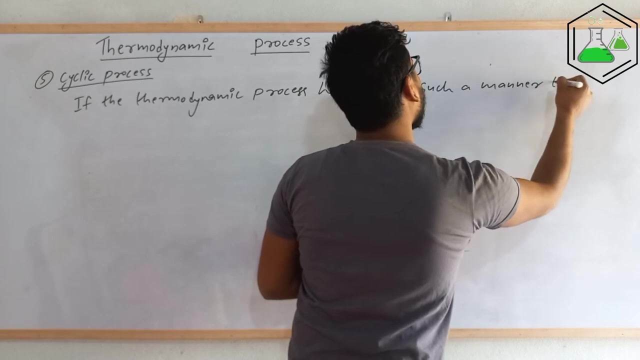 the cyclic process. if a thermodynamic process happens in such a way that, after a series of change of state, the system comes back to its original state, then that type of process is called the cyclic process. let me write that if the thermodynamic process happens, happens in such a manner that in such a manner that 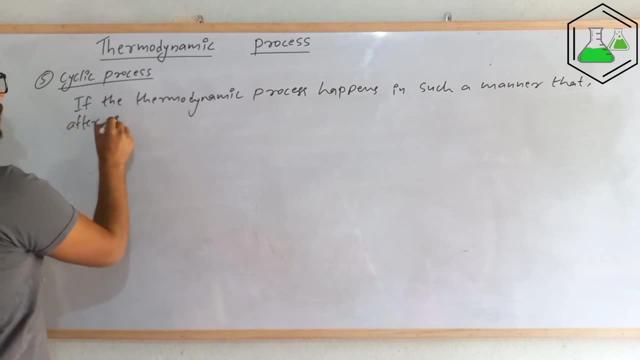 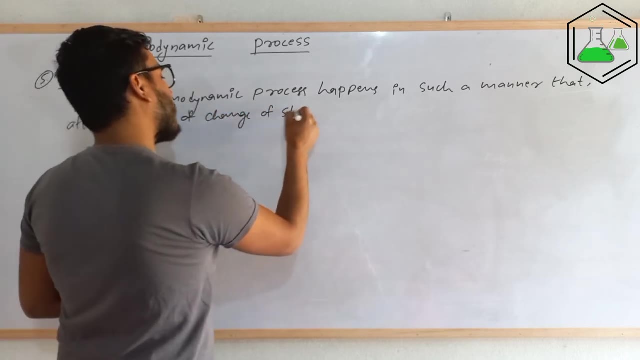 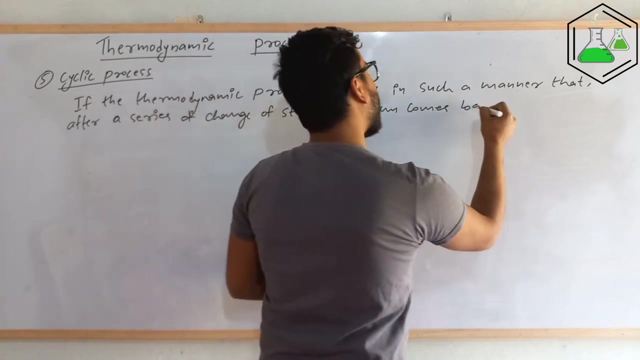 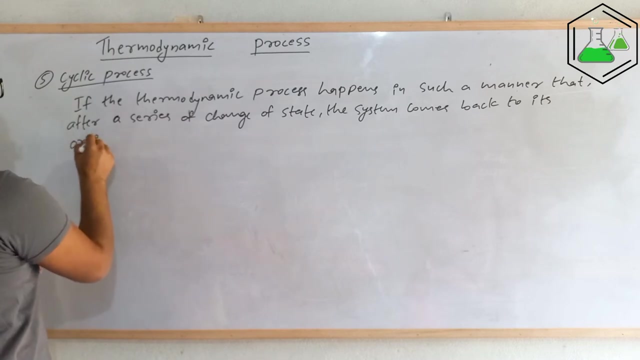 after a series of change of state, the system comes back to its original state, then that happens in such a way that, after a series of change of state, the system comes back to its original state. if a thermodynamic process happens in this fashion, according to the 刻ic, close your Pay. 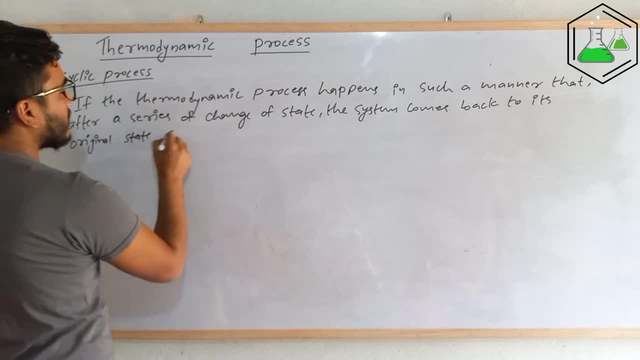 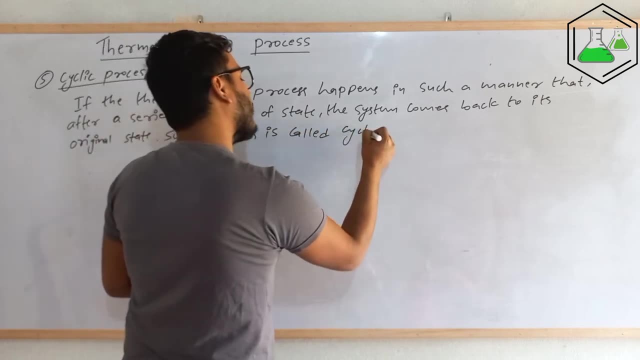 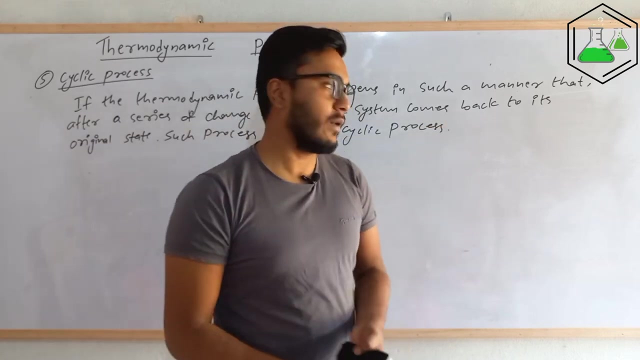 ' Let's see the next phase. such process is called cyclic process, since the process is based on the channel timeless cyclic process and this is the same process that happens in Carnot cycle as well. Graphically, if we see, we get a graph like this: 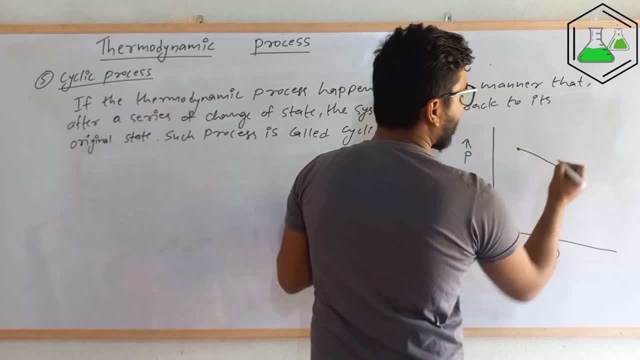 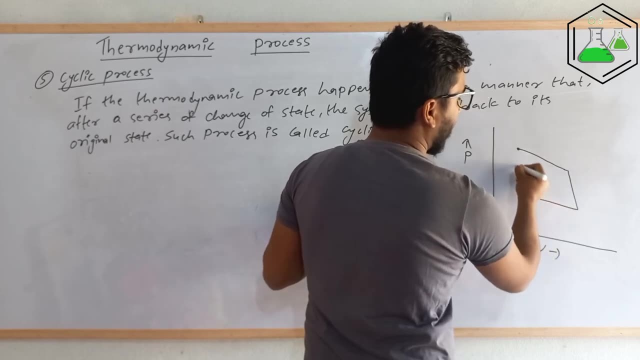 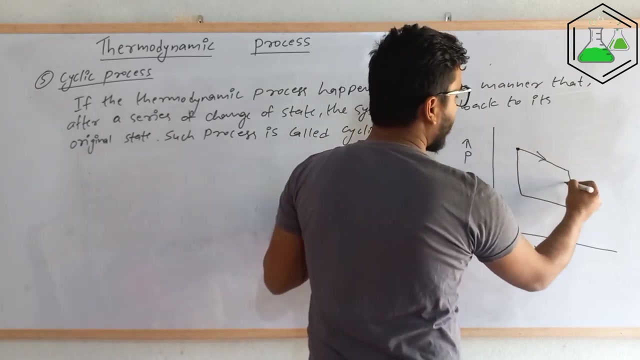 Suppose this is the starting point, then either by expansion or compression, Let's We get a graph like this, then we get another graph, another graph and finally this- Remember, this- ends on the same state at it was originally. So the process might happen in this way: it starts from here and after a CG series of change of its state. 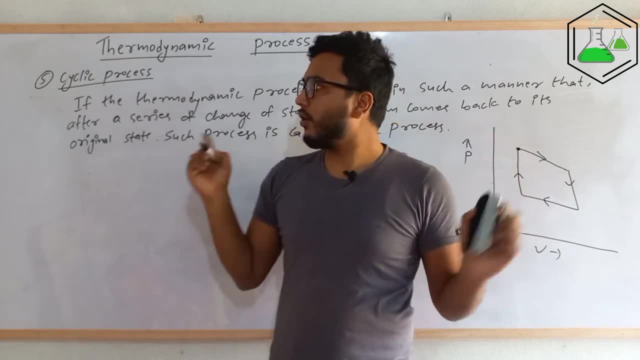 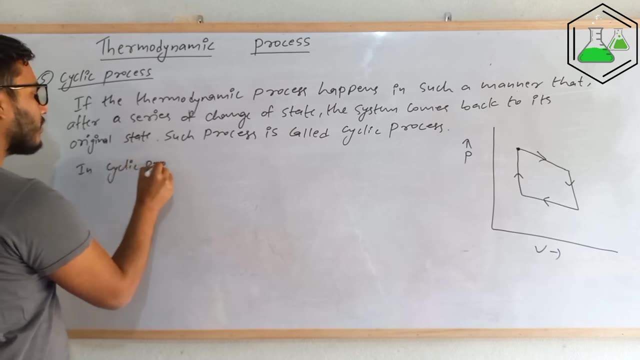 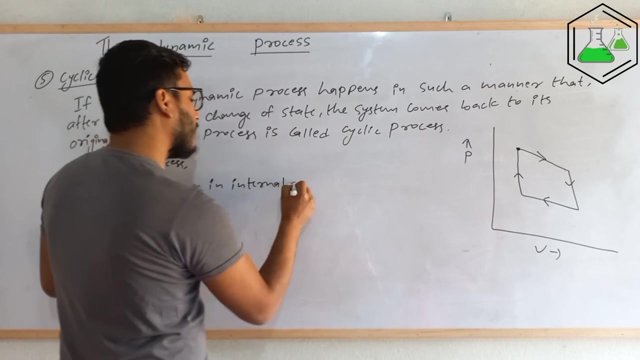 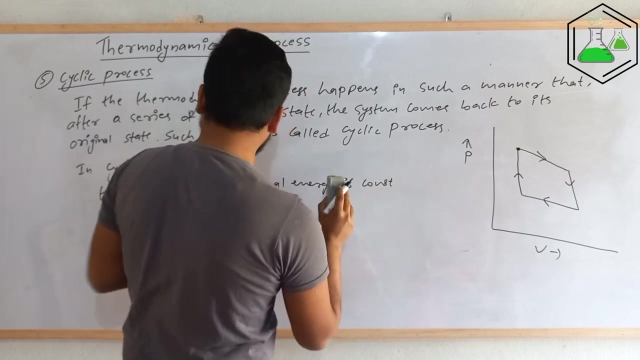 It reaches there again. So this type of process is called the cyclic process. now, in cyclic process, in cyclic process, The total, the total Energy, sorry, the total change in change in internal energy, internal energy of the system is constant, Is constant, sorry. the total change in internal energy is zero. 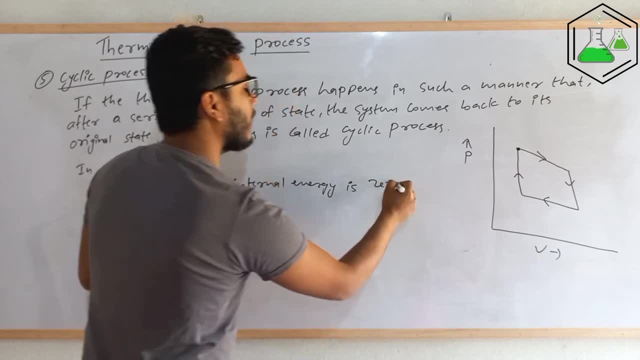 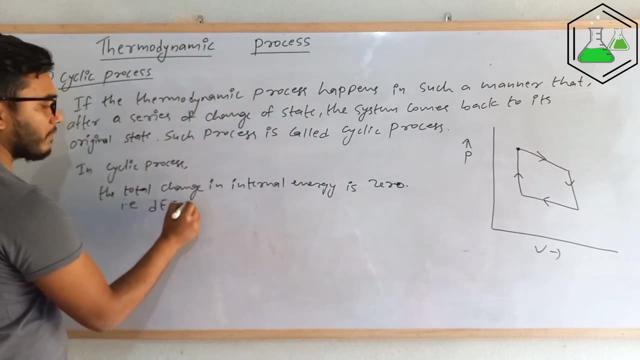 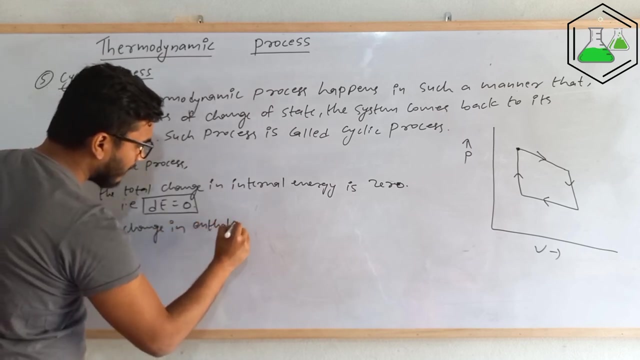 Is zero. that means in a complete cycle the internal energy will be constant. that is, De will be equal to how much zero change in internal energy will be zero. similarly, one more Thing happened over there. That is the change, the change in enthalpy. Enthalpy is also. 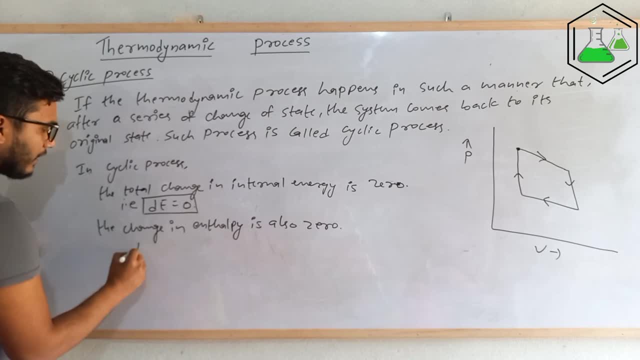 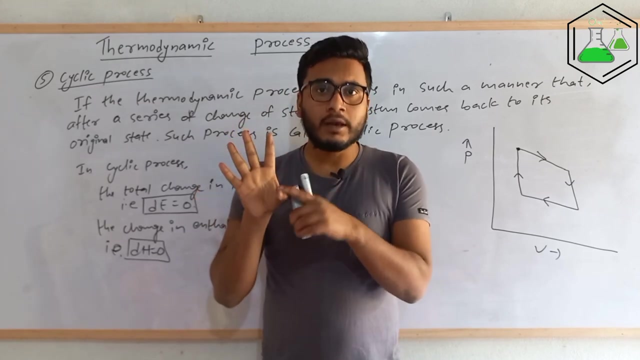 Zero. so in complete process the change in enthalpy will also be zero. So these are the two things that happen in a cyclic process. So in this video we talked about five process. They are: isothermal, isobaric, isochoric, adiabatic and cyclic process.